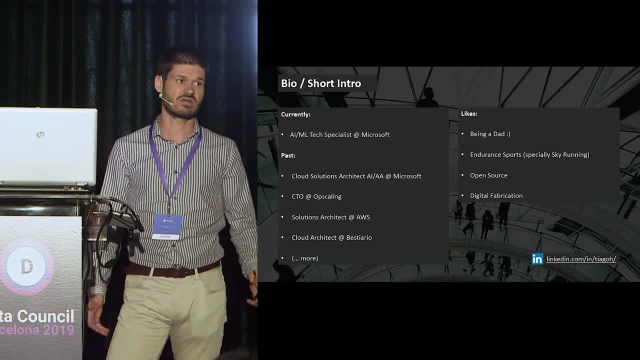 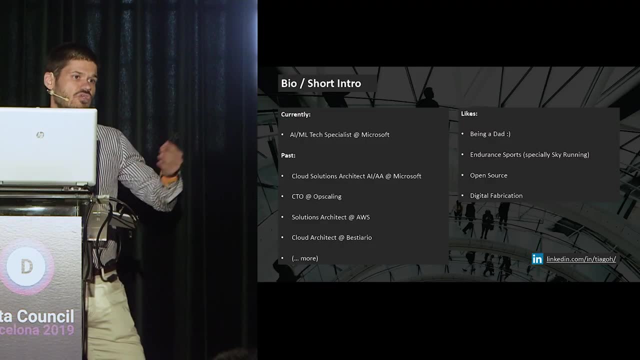 to make their data science process And teams a bit more agile, or helping them to deliver best business value or more agility, especially as you grow in your data science practice, to make it more effective and also possible at scale. That's a little bit the idea. 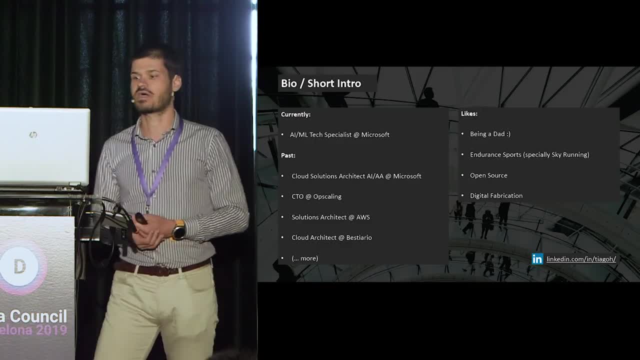 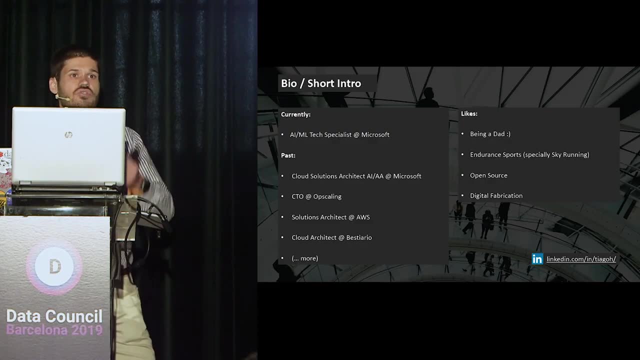 I must tell you there is a few things in my presentation that you might don't agree might be chalked. That's great. I invite you to drop me an email or connect with me on LinkedIn And, as Jordi mentioned, in the end, there's also some time that you can make any questions and discuss different perspectives. 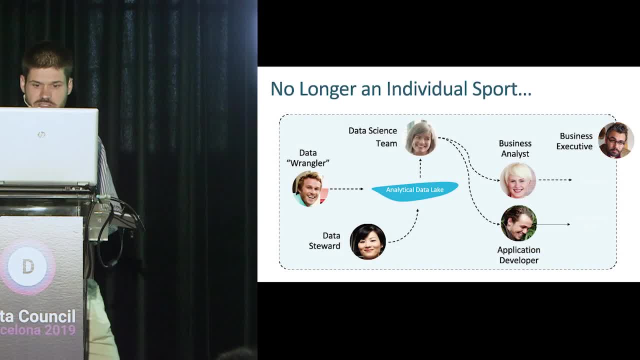 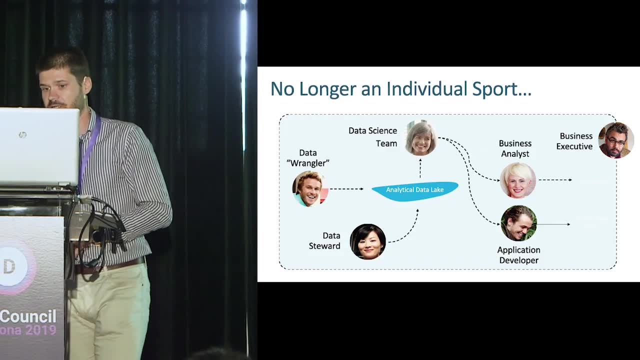 But those are just a few things, A few things that I wanted to highlight. So the first thing I see in organizations- once more large organizations, large companies- is that the last few years, of course, machine learning is not something new. 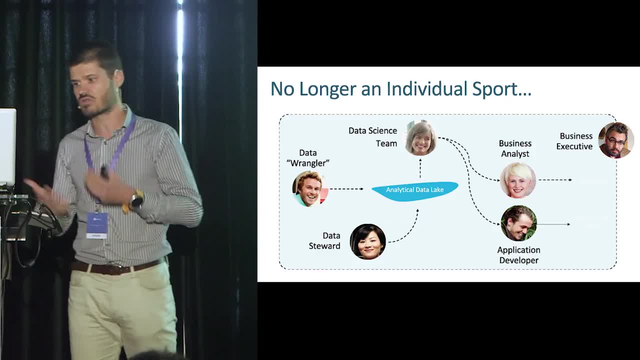 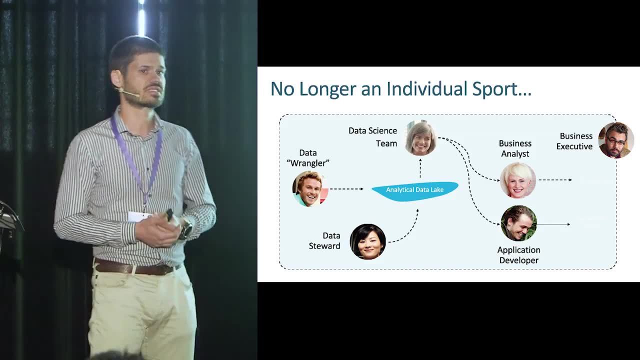 I think it's just becoming more popular, more adopted for different effects. I think cloud computing is one of them. Open source is another one. People are more skilled on that space as well. But I see there's a big trend on the data science teams, because initially data mining might have been with statisticians. 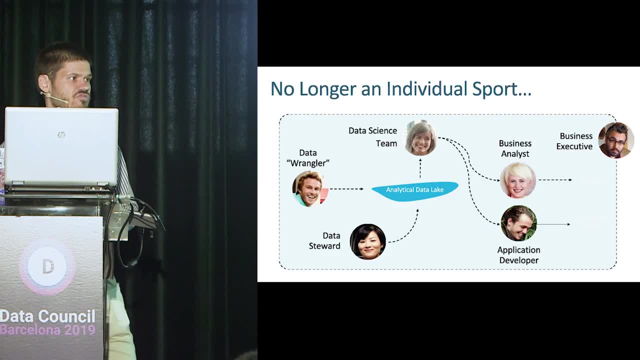 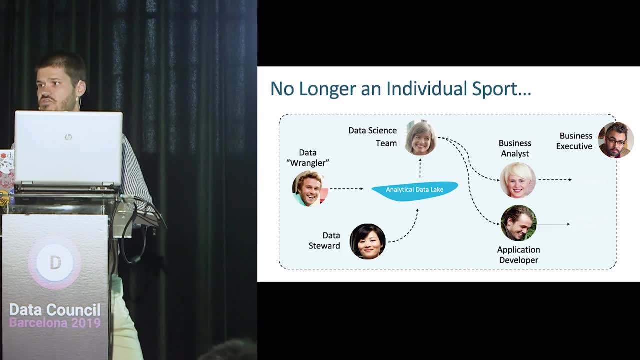 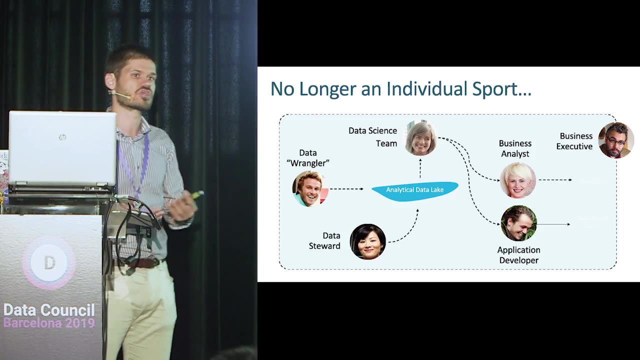 A very individual job, So people were doing a few statistical models, predictive models, on their laptop and connected, of course, with the business. But more and more I really see in the conversations with the teams I have- from chief data officer, head of analytics, data science teams and business teams- that this is really a shared sport. 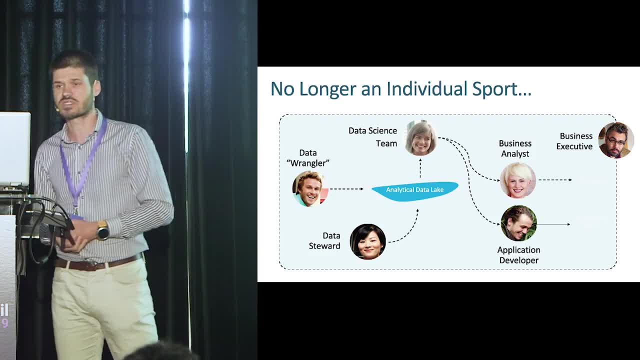 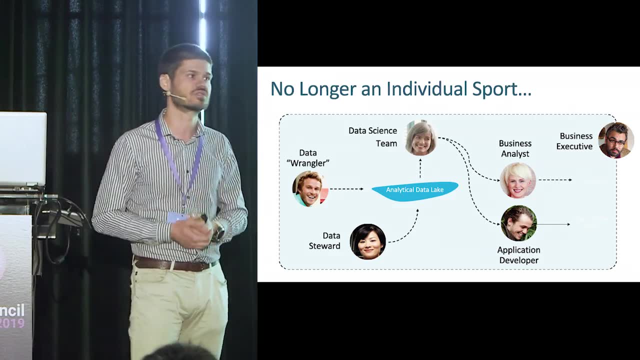 And by that that means that there's also a change in process that needs to be in place. First thing, I think, coming from top, is that of course, companies need to have a data strategy. Of course I will not, Of course I will not bother you with that topic, but that's extremely important. 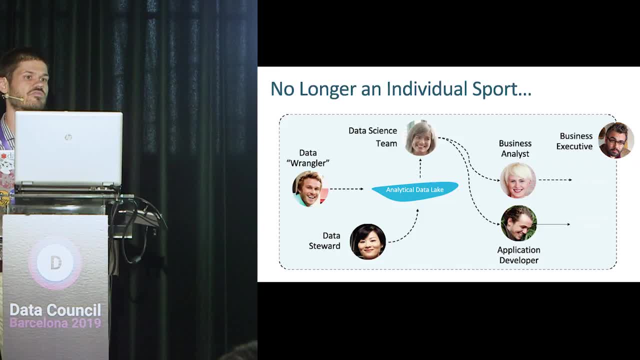 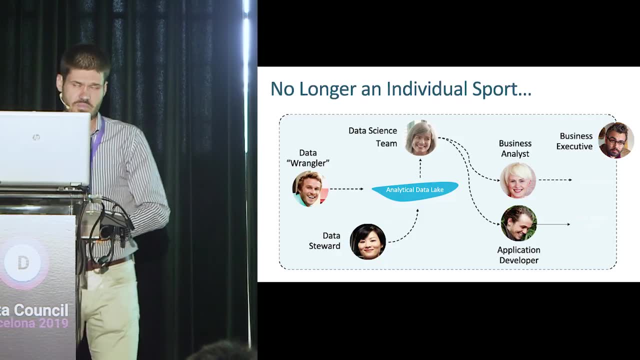 Then over time, of course, when you have data, more data needed for your business drive, let's say, a culture of data driven decisions. That's definitely what teams want to do, And then there's a few roles at play in this discussion. 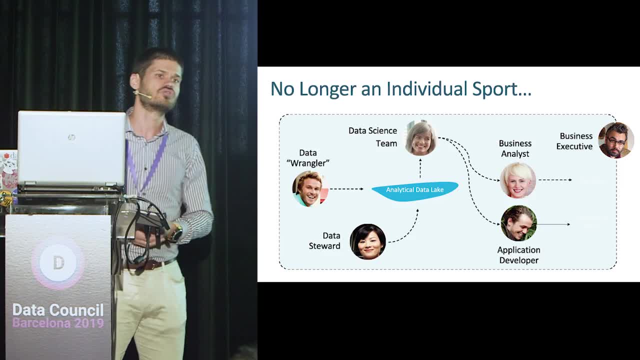 This slide is just a subset of that. Today we're going to focus most of my practical tips I want to give you are, of course, going to be focused on data scientists, But of course, as you know, there was just talk. 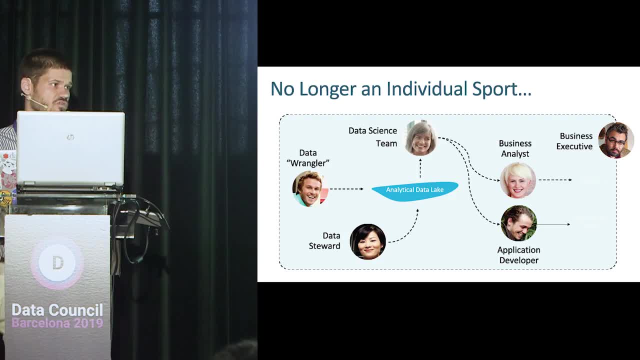 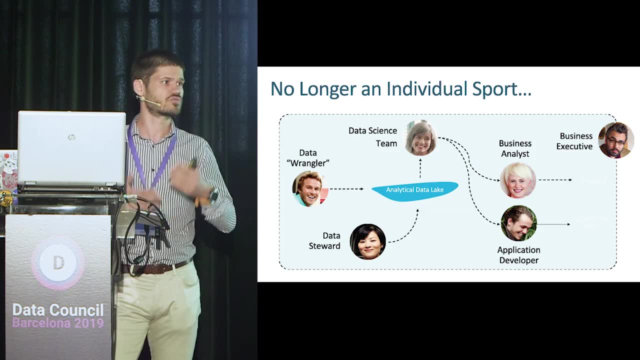 Before. as you know, there's a different track on data engineering. That's a big part of the job. before you can start to get and work with the data. I forgot to introduce myself, to ask a few questions to you so I know better who's in your team. 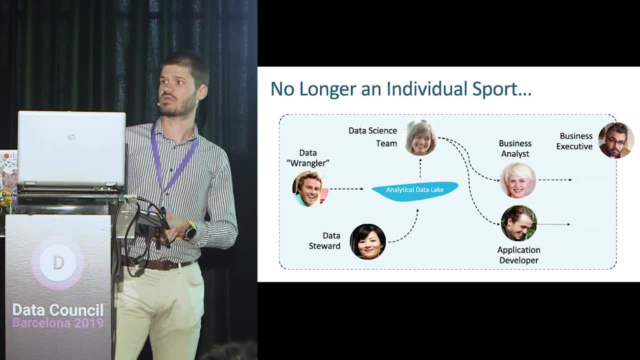 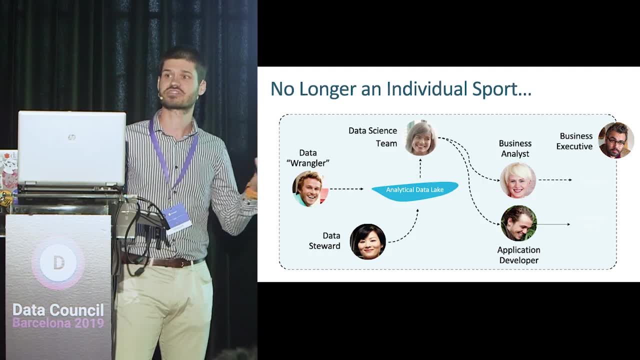 Who's the data scientist, by the way? Okay, That's close to 50%. That's great. Data engineer- Okay. Some people skipped the other track Managers, Okay. And who works for a startup? Who works for a large enterprise? 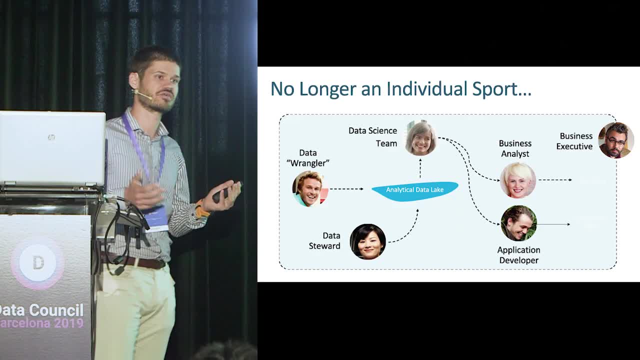 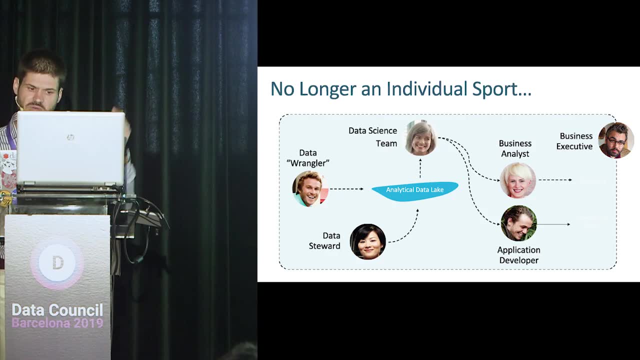 Organizations. I feel like 50% on all my questions. Okay, That's great. So, like I said, there's a lot of processes that need to be in place. In the end of my presentation, I have a link to one of the options to adopt a process for data science from end to end, because it's not just about one use case. 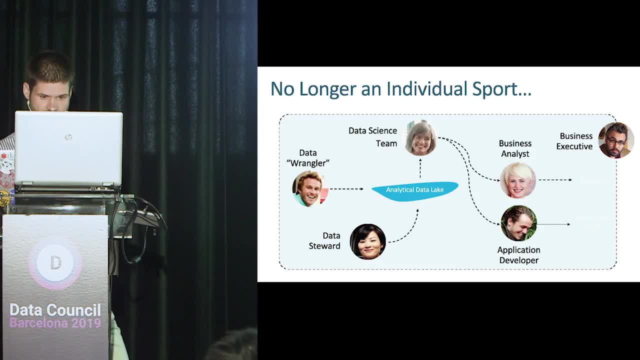 It's about getting the business with new processes and adopting them. So, from now on, without going into detail with all the roles you see in these slides, it's really about what I think you can do practically to improve your data science practices. 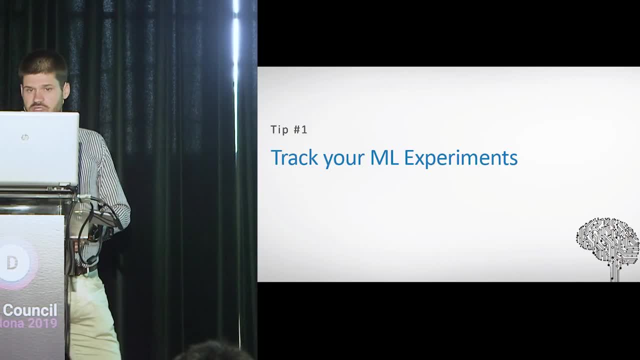 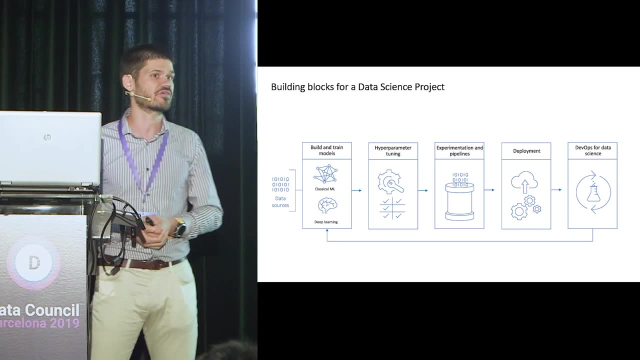 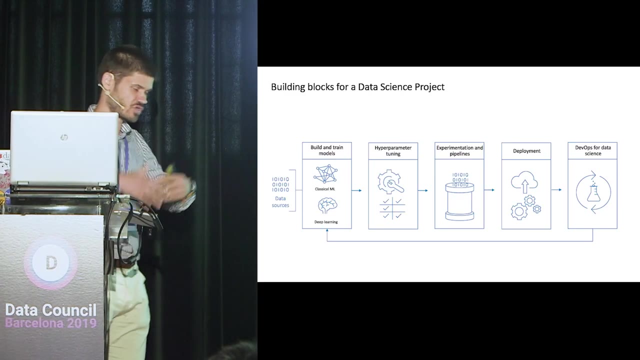 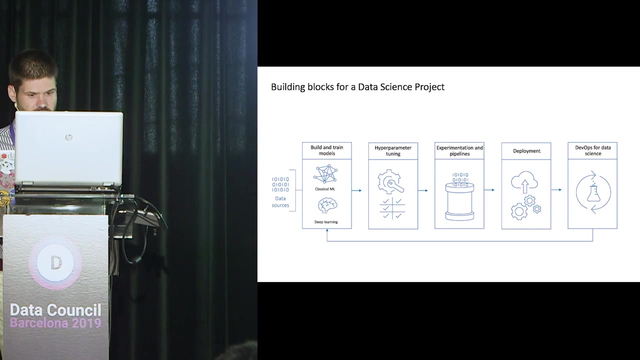 Just five tips. Hopefully they will fit in half an hour and there is some demos in the middle. First one: of course, data science is extremely interactive job. right, You start with the business problem. You get some data, You start to build models with your favorite programming language, your favorite frameworks, sometimes using more sophisticated methods as deep learning. but you don't need to. 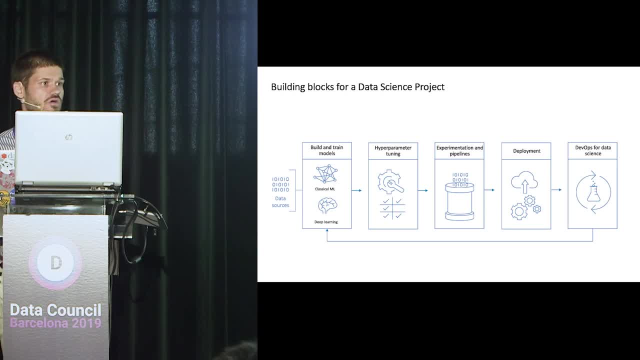 And, of course, most of the time it's really about tuning your models, the parameters, Do more experimentation, Create machine learning pipelines, And then, of course, that doesn't finish. That's why I had a slide before about teams. 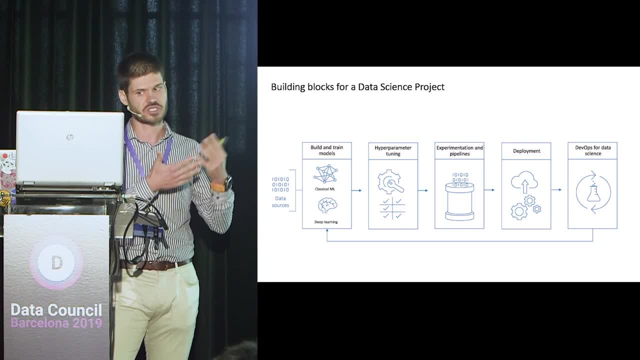 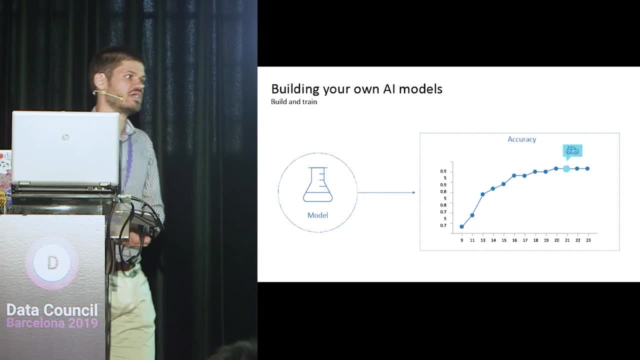 When you have a pretty model, you need to have a process to deploy it into production and get it integrated with your applications and end users. Okay, So one of the things I've seen that I think it's very important, especially when it's not one person. 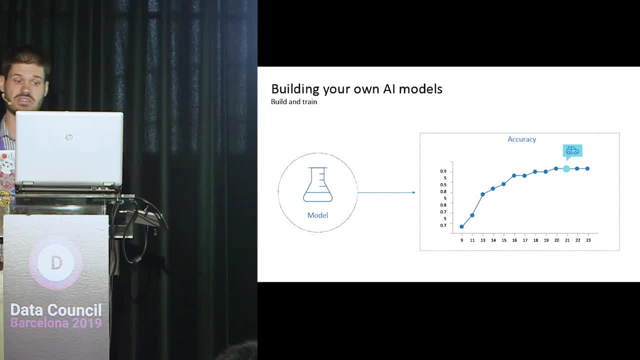 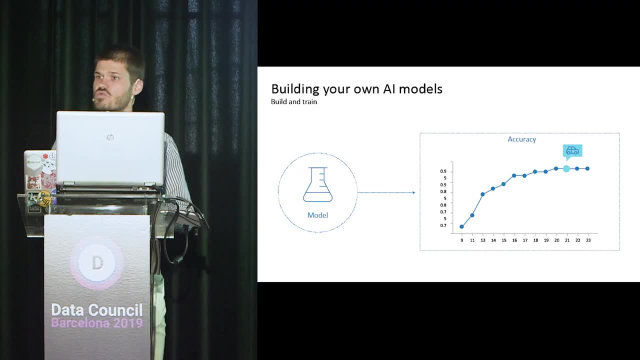 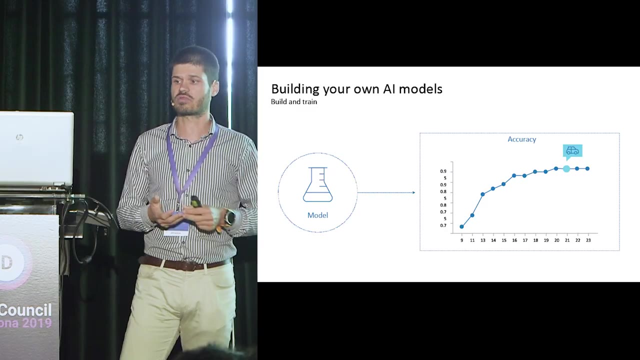 It's five, ten people doing data science in a company, sometimes across different departments. Some people might be doing data science, Some people might be doing pure code, Some people might be doing more visual things. It's really about every time you run machine learning experiments or every time you do some different, trying a new algorithm, trying new parameters- make sure that those experiments are tracked. 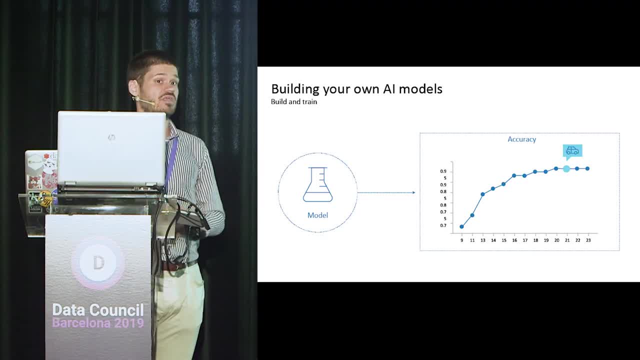 Okay, Because first, you have a record of everything that is happening in your data science practice, especially when you have a team, when you're doing different projects. That's really important. And second, because you want to find what is better over time. 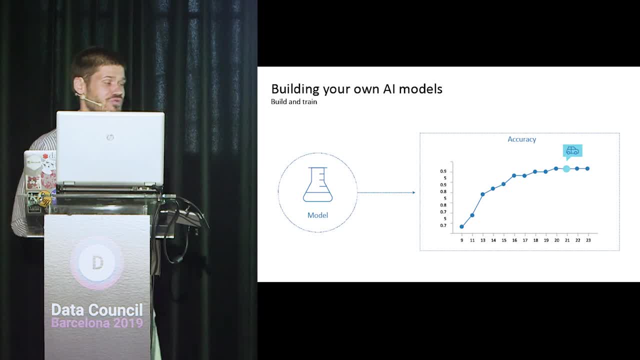 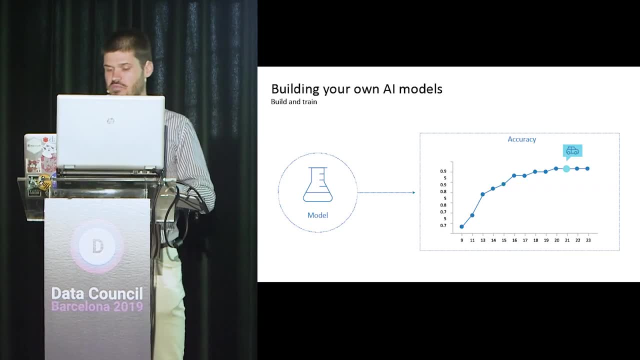 And sometimes you don't remember exactly how did you achieve that. I've seen people doing that, So that's also for reproducibility. So some point in time you want to know how did you achieve some result with which parameters? Let me show you a very simple example what it means. 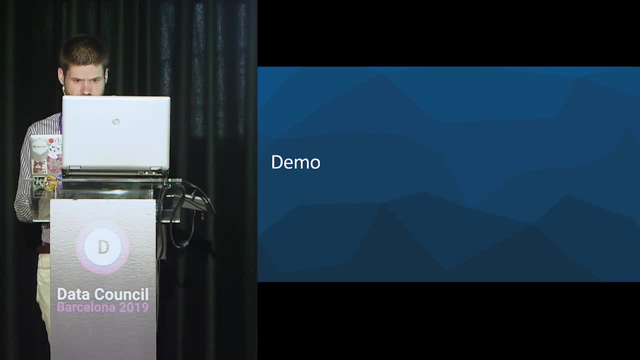 Of course, using the cloud. In this case. it's interesting because I'm still using my laptop. As you can see, this is Jupiter on my laptop, So I'm still running locally. The only thing I'm doing is importing a small SDK- Python SDK in this case. 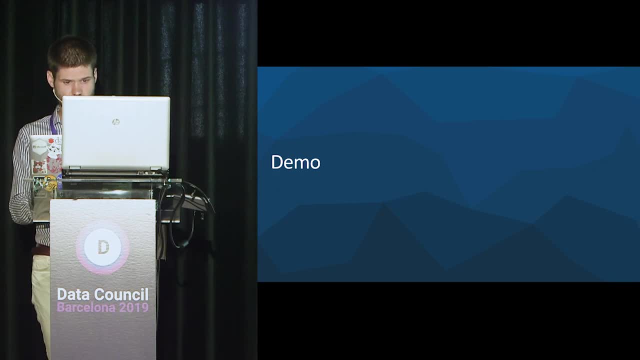 Just checking the version Connecting to my workspace. That's a service that we leverage in Azure for Azure machine learning. Those are just some details behind the scenes that are not relevant. Sorry, There was this one. actually, Those are just the configuration parts. 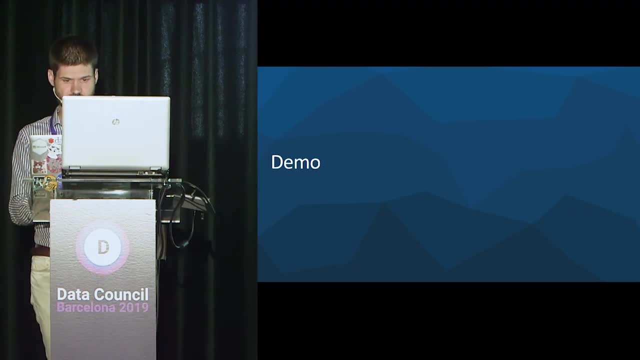 Then what I'm doing is I'm running an experiment. Sorry, This is really the right one. Okay, Let's start with this one For sure. Okay, Now it's in the right place. Okay, So I'm saying I'm doing a training. 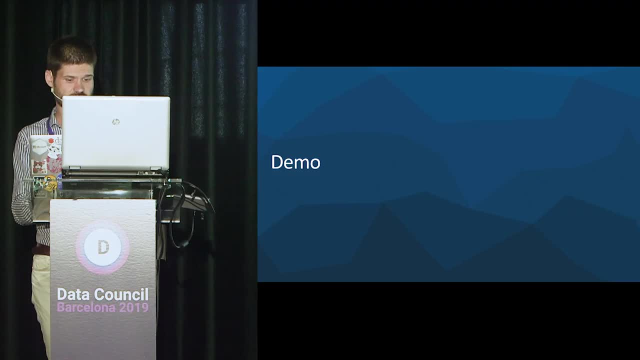 I'm just experiment name and locally This is my train file, Not going to bother with the details. This is standard for data scientists, data set from scikit-learn. This is just my training file. I have just an auxiliary library. Then I'm saying I want to use my laptop environment. 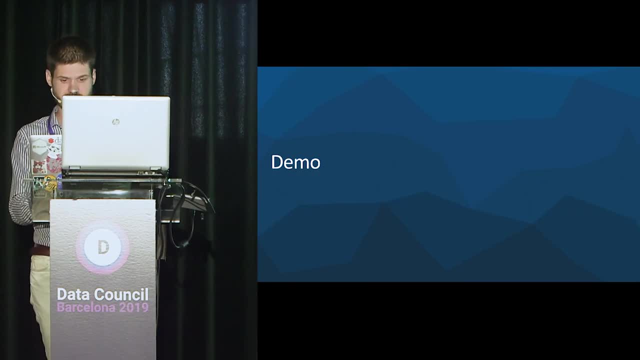 So in this case, of course, conda To have an easier life, Then I'm just saying that I want to submit this to my environment Once more. this is my laptop. I don't need to get out of it. 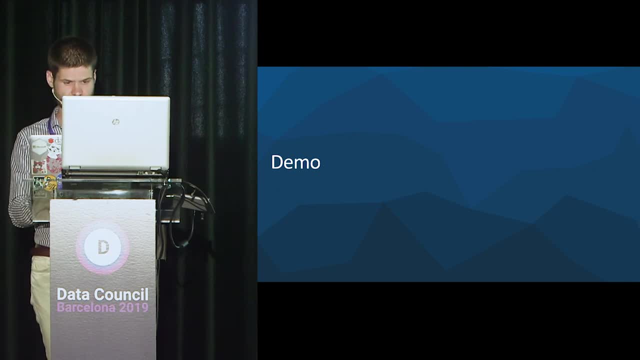 I will be running my experiment. Give it a few seconds. Of course it's a simple model, And now I can even see how it iterates over time. So you can see this is really fast because it's a simple problem. 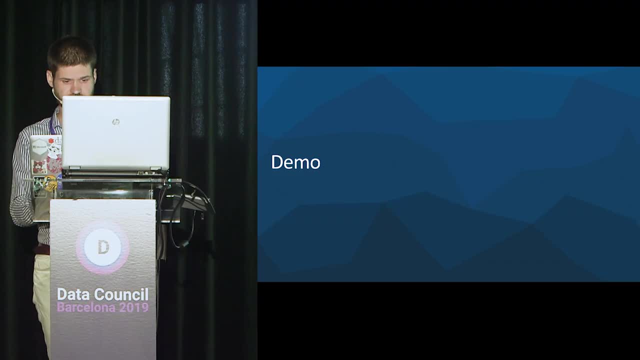 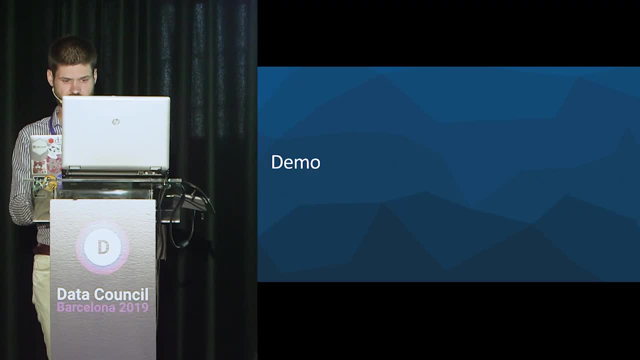 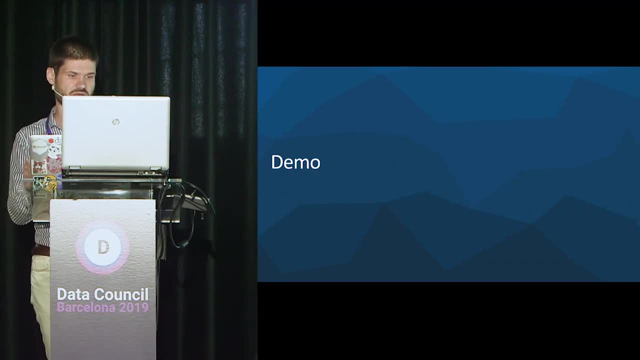 Okay, This is nice. I already see what is happening here. But back to my original idea, The idea that you have a place where you can loss all your experiments that you have running. So what I'm doing now is wiping to a graphical view on Azure. So what I'm doing now is wiping to a graphical view on Azure. So what I'm doing now is basiallly tis all the runs I've ran in my laptop. right now I have a graphical way to see, over time, everything that happened behind the scenes. 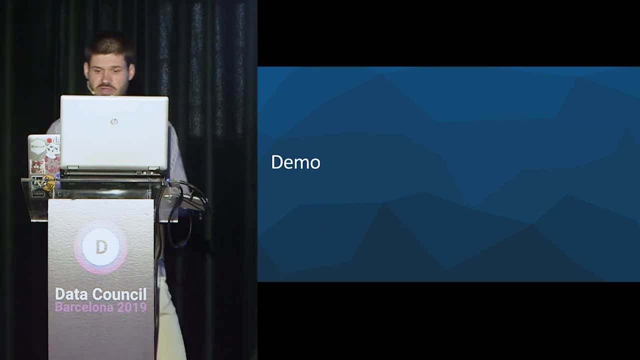 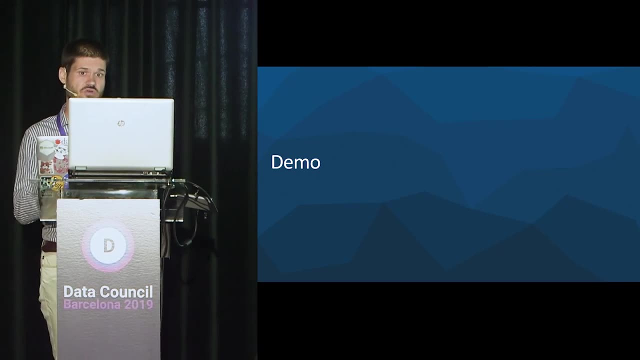 I have a graphical way to see, over time, everything that happened behind the scenes. Okay, In this case I did just this much tactical work. Okay, swapping to a graphical view on Azure, that basically all the runs I've run in my laptop. 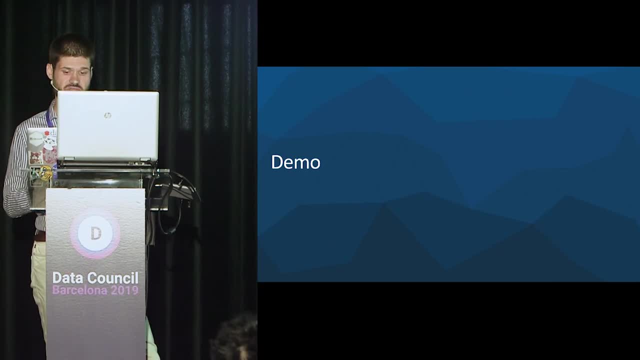 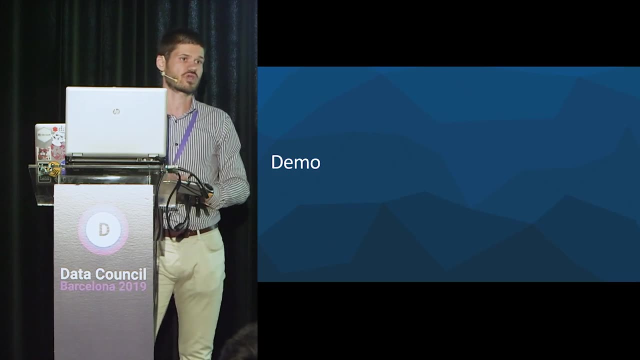 right now, I have a graphical way to see, over time, everything that happened behind the scenes. Okay, In this case I did just a few iterations, but I can now already see what are the key metrics I want to track and, over time, how they perform. Once more, this is a very small. 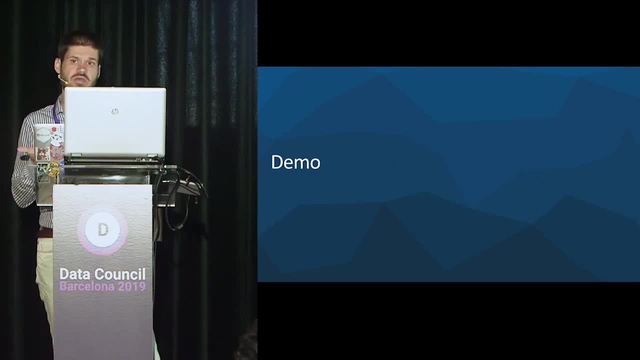 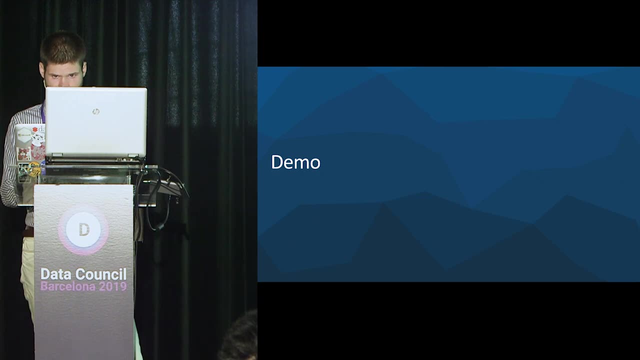 example, and I'm going to run something a bit more complicated, but that's already a best practice. Secondly, Let me find the right notebook this time at the beginning. Secondly, I'm doing exactly the same thing, but of course we said that we want to leverage. 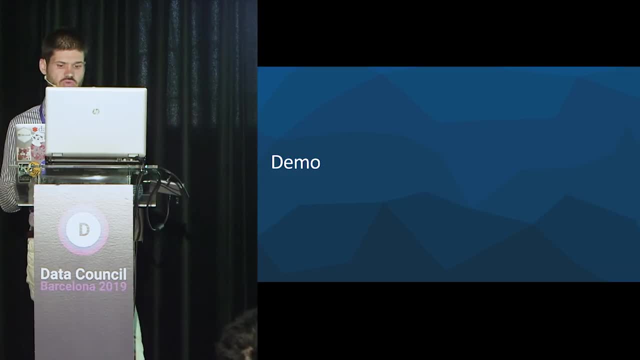 the clouds and still give it the principle of tracking experiments. What I'm doing now is running a simulation experiment but saying I want to have some extra power. Of course my laptop has a limit of CPUs, of course, and memory. I want something bigger. I want a bigger virtual machine in. 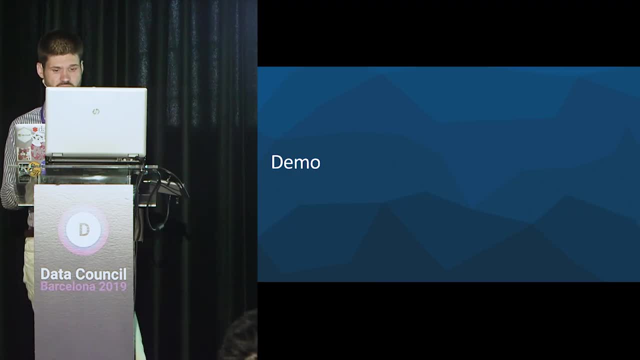 the cloud. So I'm creating a new experiment that I call it train on remote VM. I'm passing all the parameters, getting the data sets. I want to read the details Once more. I have a file with my training script, very similar to the previous ones, Then I'm attaching it. 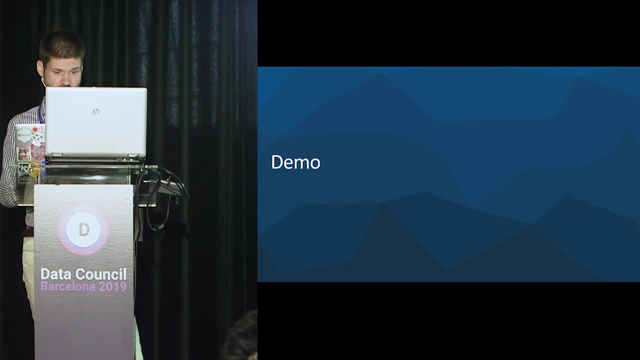 to the machine running it. I've run it this morning so I can save some minutes in the presentation. As you can see, these are all the details of alpha MSC and all my conda packages within the environment. When it's finished we can go back to the portal, Not. 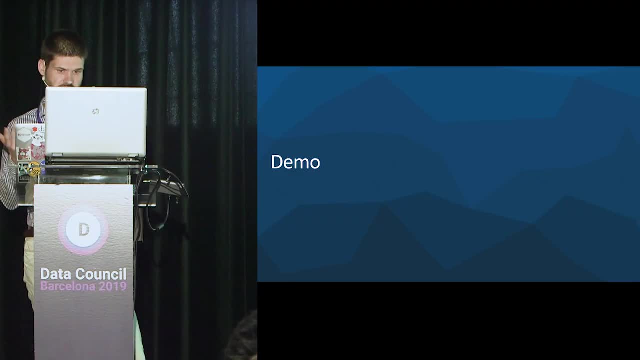 yet that one. And now, in this case, as you can see, this one took, I think, five seconds per iteration. Our credentials have expired. This is what happens when you change IPs. Give it a second. Okay, As you can see. now I see for every run in my code. of course I'm swapping parameters. 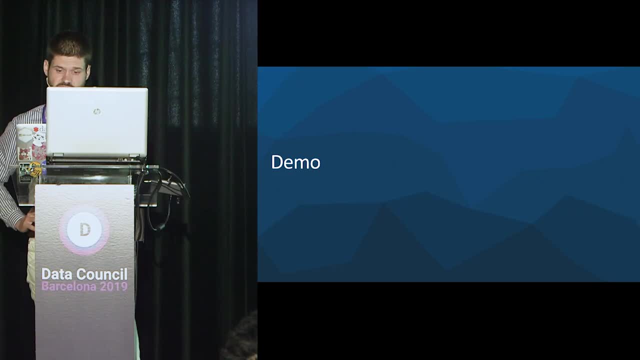 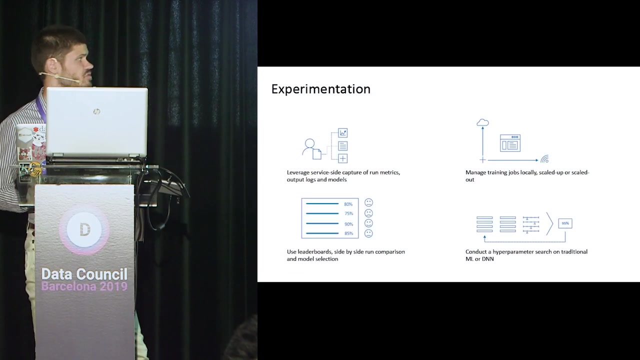 how long it takes and what was the values I'm tracking for MSC So I can very easily come here and see which one had the lower MSC. Okay, So this was my first tip. As you can see, using Azure Machine Learning or potentially, 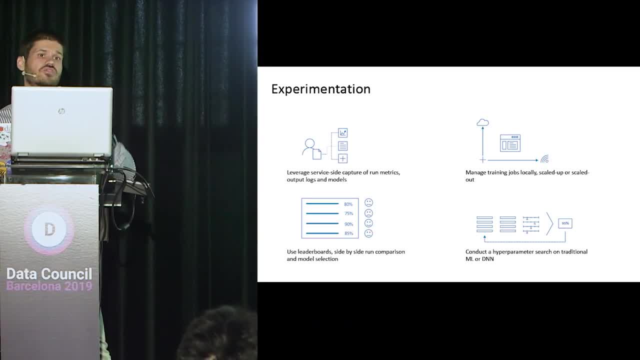 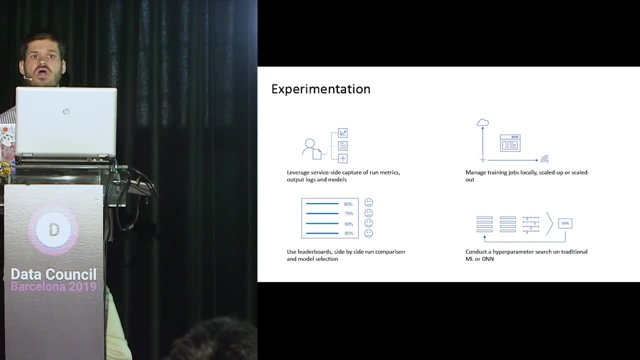 other ways. you have a centralized place where you just log your code, no matter where you're running on your laptop in a bigger virtual machine with CPUs, GPUs. you're just able to track what you're doing and what your team is doing. Okay, So that's one first tip. I 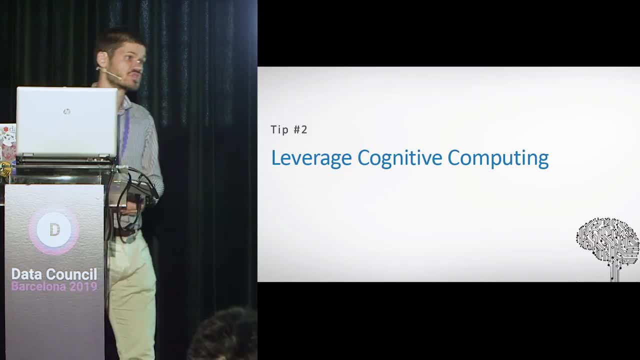 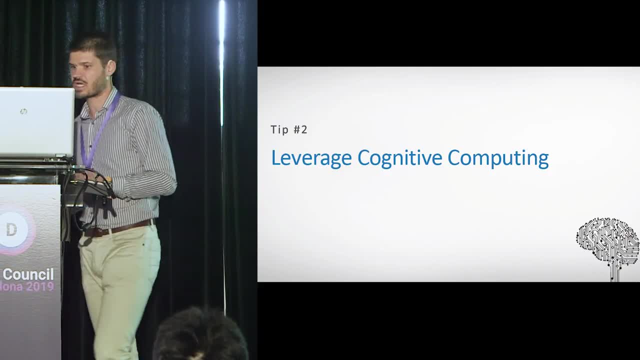 how to do it. So I'm going to show you how to do it. So I'm going to show you how to do it, Even for professional data scientists, which might be more than 50% of this room- is to leverage what you already have out of the box in the cloud. So there's this concept. 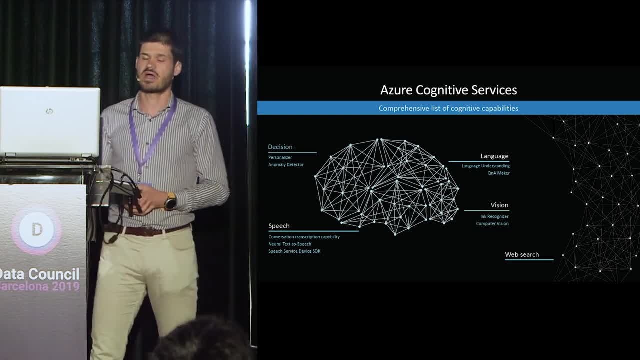 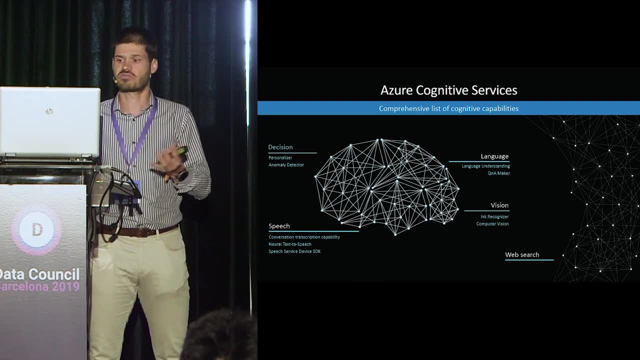 of cognitive computing, which is basically the idea, is to build APIs, pre-trained models that are consumed as RESTful APIs, where we embed some of the capabilities of humans. That's what it's called cognitive right. So you have vision capabilities speaking. 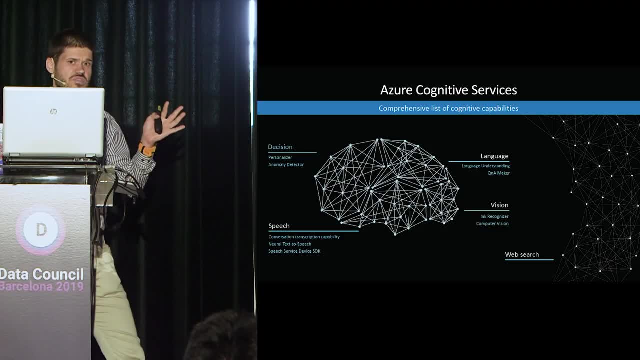 capabilities, understanding capabilities. What you see here is just a very small subset of human capabilities, So you have vision capabilities, speaking capabilities, understanding of what is available as a cognitive service, as we call them, in Azure Cloud, But basically it's the idea of a model that has been trained. Most of them are deep neural networks trained. 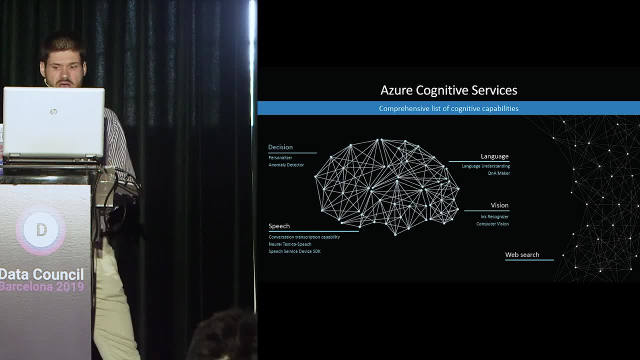 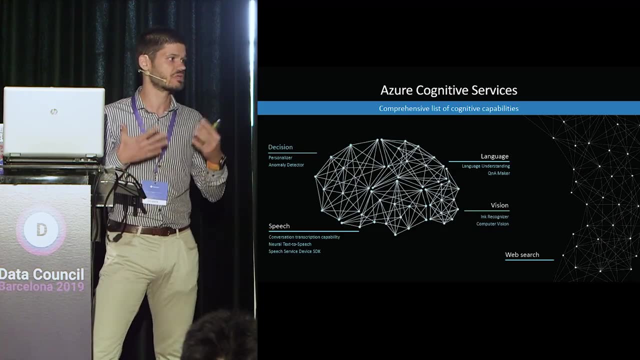 with a very large data set to solve one or multiple problems and you can just consume them. Why I mention this to professional data scientists? Because sometimes, when you're starting a small project or a small problem that you want to fix, sometimes it's not worth. 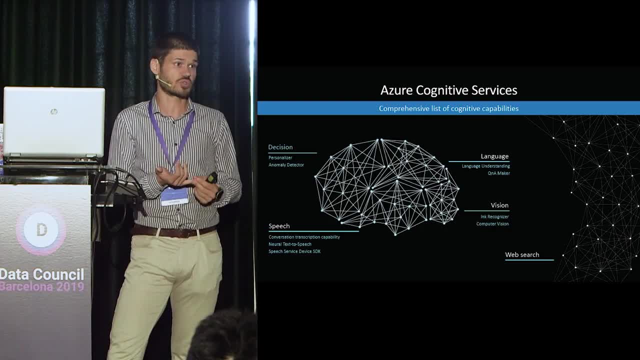 the time or the investment to train your full model from scratch, because you just want to validate that you can achieve something or you don't have enough time to do it. So you have data to train that model. So one way is maybe start with those APIs More and 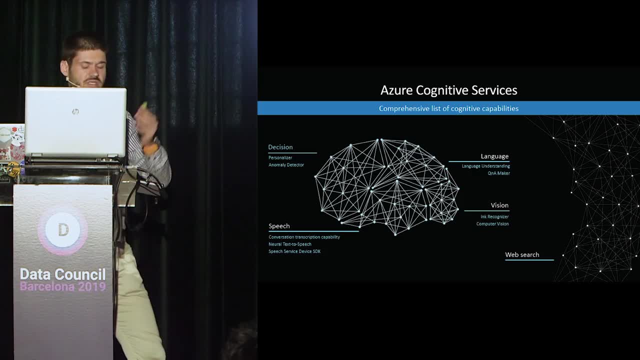 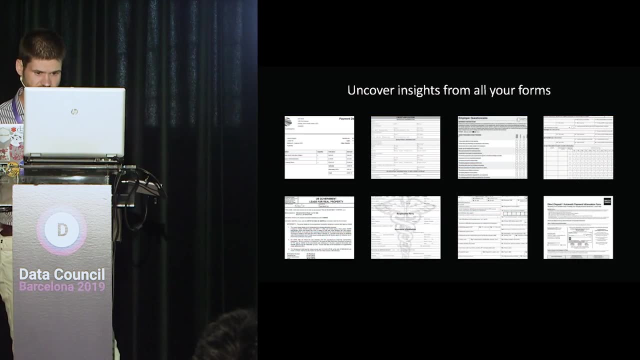 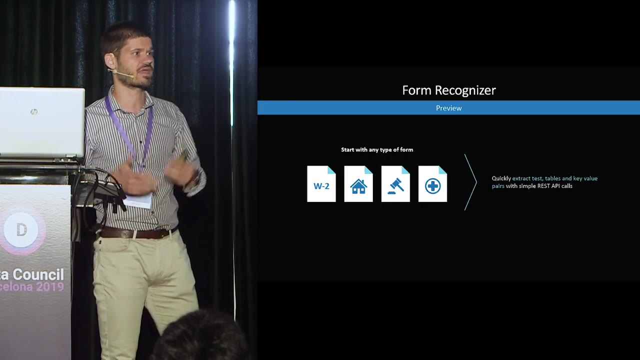 more. over time those APIs start to be more customizable, So you can basically modify the external layers of the neural network. So one example of a cognitive service is for forms. So you have a set of forms like medical checkup, text declaration or any kind of 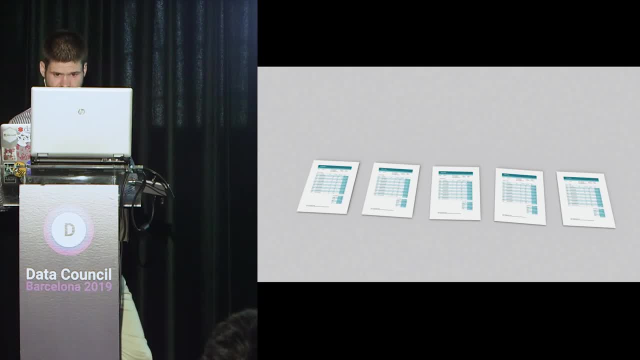 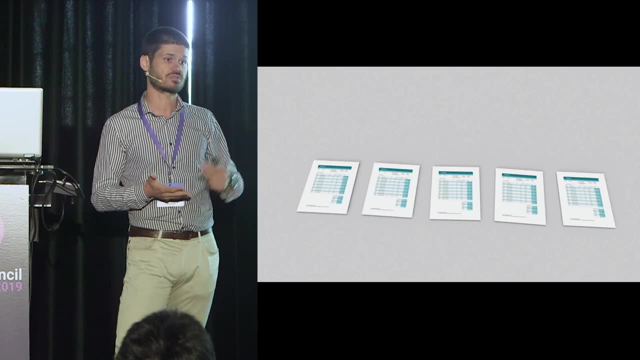 document actually And basically using one of those cognitive services. I know it's a good idea Basically just sending the document, the PDF, there. It just scans, It detects tables. This guy is an invoice, Could be also a receipt of a bill, And basically just tries to figure. 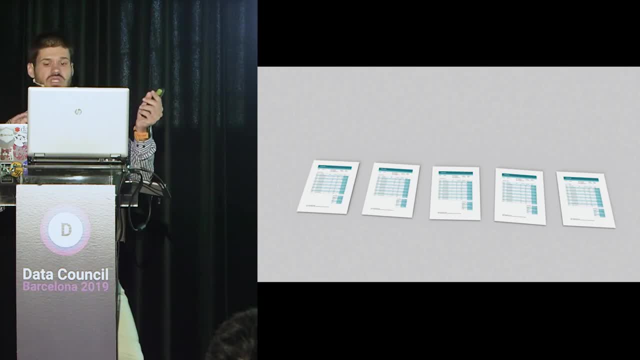 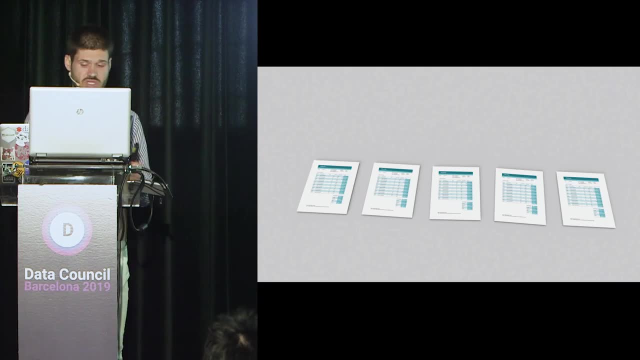 out what's the information there and extract it as a JSON, So you know exactly what is the table there, what fields and so on. That becomes unstructured into structure. Okay, Once more, think about doing all this from scratch in a data science project. Two more: 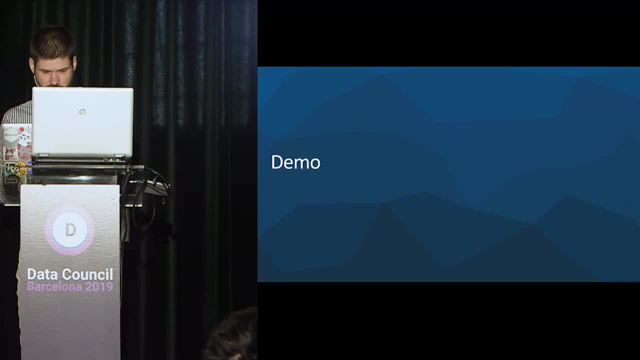 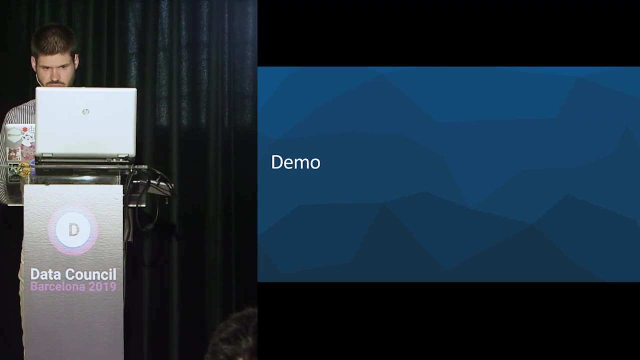 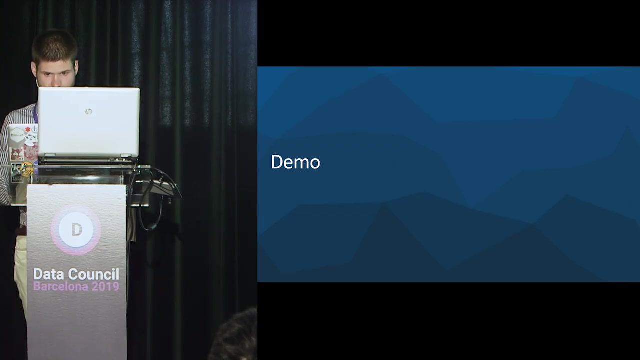 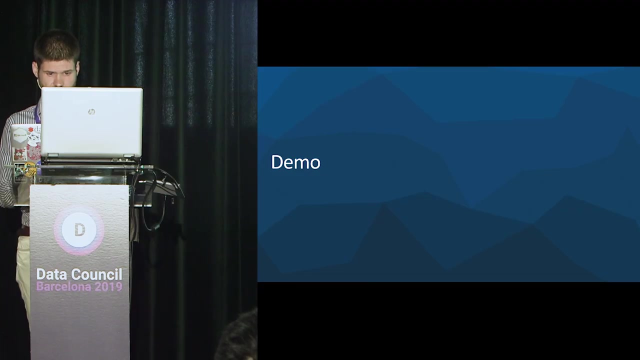 things. I wanted to show you where you can leverage cognitive computing. So these are the five categories I mentioned. Vision is one of them. So a few things that you can do with this service is, for example, analyze an image. Okay, In this case I'm 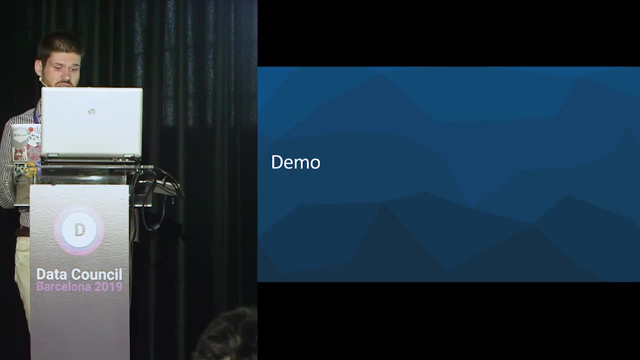 seeing a picture of a scene. It's detecting people. It's detecting there is a way in a train. So I said: okay, why don't we try with this? Why don't we try with this? Why don't we try it a different way? Okay, So I went to my browser and I saw there was some nice. 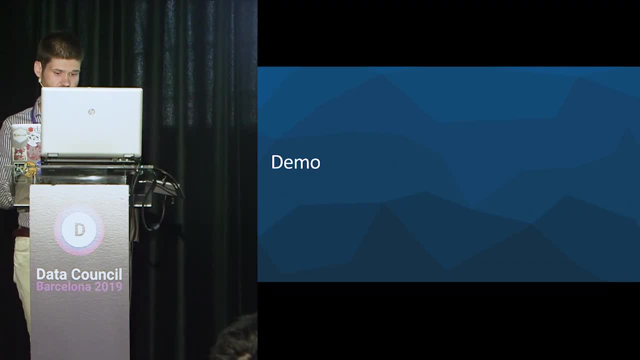 picture of the day of penguins, So I took a screenshot of that picture and see how it performs there. This is the right one. Okay, Same picture I showed you. I'm sending it to the cognitive service So it's able to identify a lot more things that I mentioned. 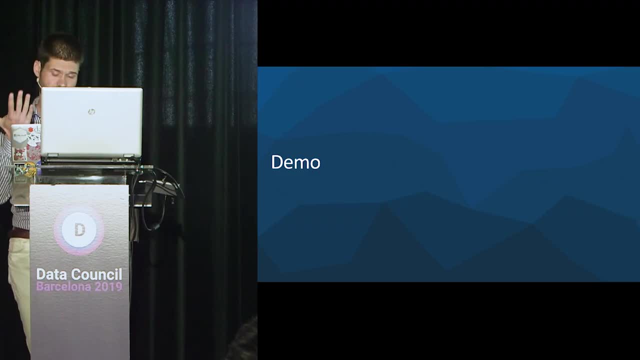 to you. It can also identify people, their emotions, their gender, their age, the position of the body. There's a lot more things it can detect, But in this case I'm just sending one picture I just found this morning in my laptop, if the connection stays with. 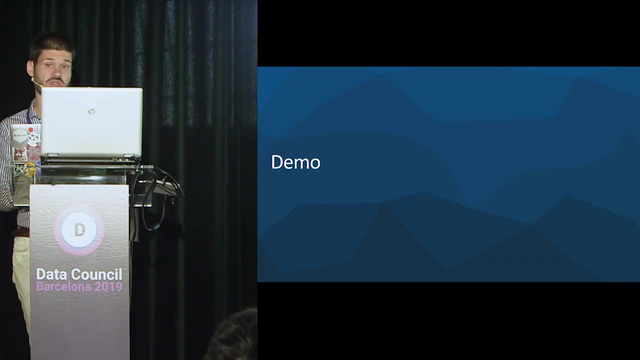 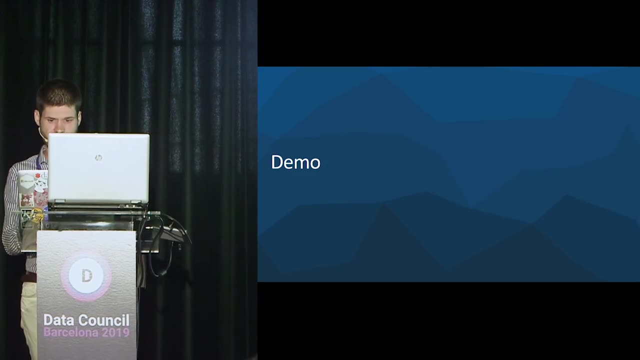 me okay. as you can see, it detected actually penguins, so it's actually trying to identify some objects and not just the penguins. of course you have the bounding boxes of that and you have a few keywords: animal, outdoor, snow, group, bird and so on. so that's actually pretty good. second example I wanted to show you. 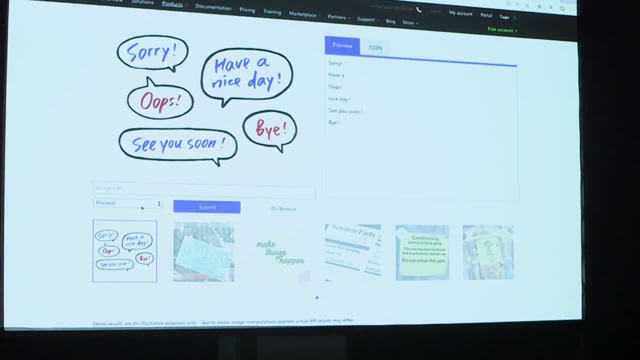 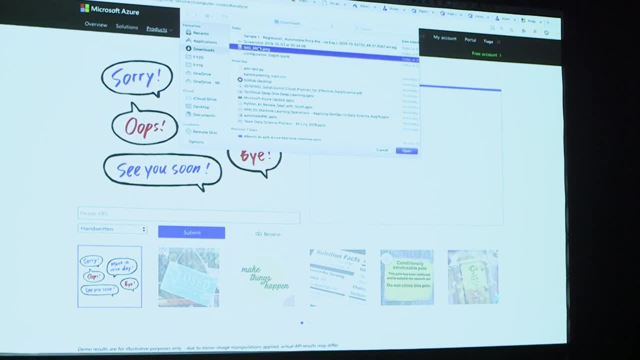 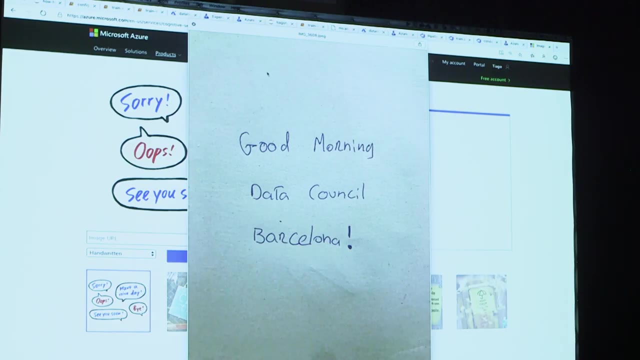 is, I think, a pretty complicated data science problem, which is detects and written text. okay, I actually been in a few projects with companies, with data scientists, to write them from scratch and they are not easy to tackle. so this morning I just wrote this with my handwritten, which is not the most nice. 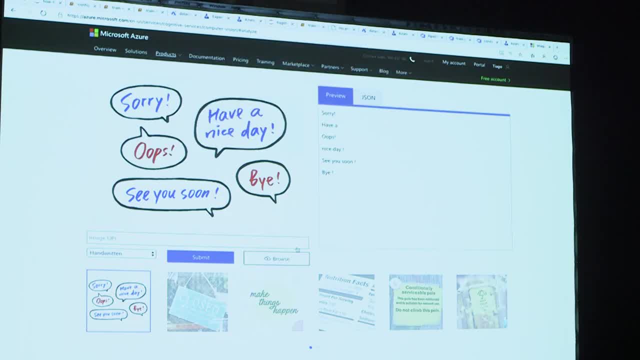 looking one, so, but it's mine. so what I'm doing is I'm just sending this to these API and saying: this is handwritten and, as you can see, even though I don't have the most nice looking handwritten, it detects exactly what I've wrote. it's. 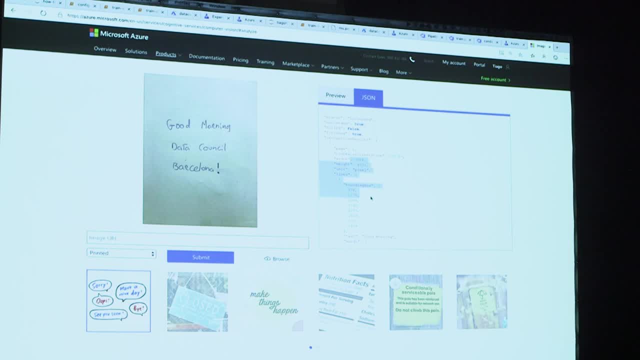 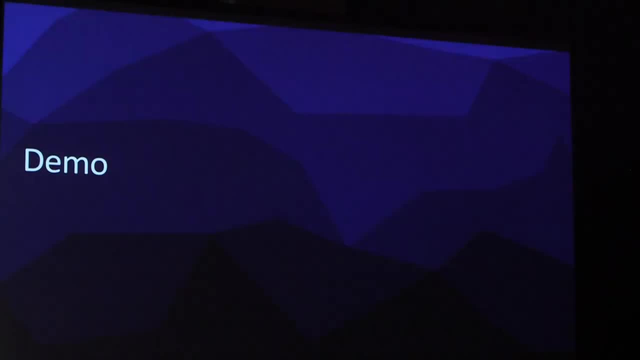 more. the result is adjacent. you can even find the location of each word with the bounding box and so on. so those are just a few examples. there is a lot more of cognitive services I wanted to show you because, once more, sometimes it's not worth to start from building your models from scratch, just like leverage things. 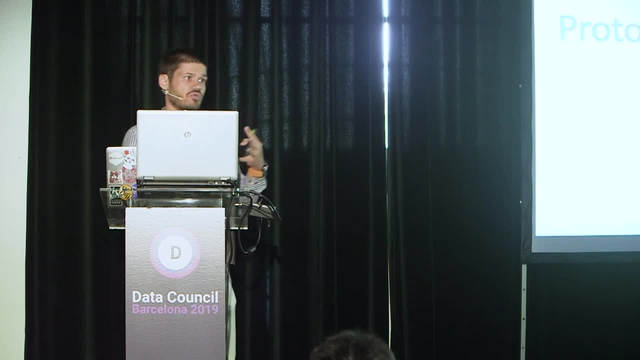 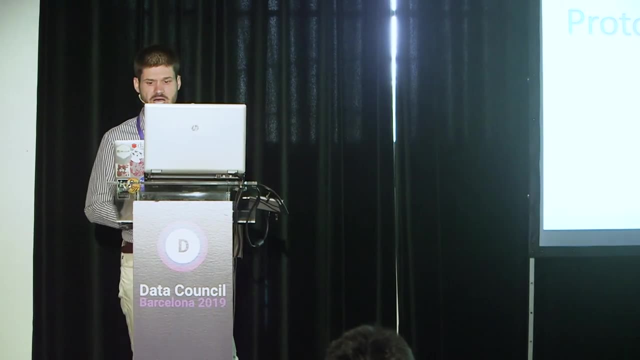 that are pre-trained and combine them with your your own train and build them into your data science pipeline. same thing for text analytics. there's a couple of good one, translation, and so on. okay, next one I want to mention to you is, even though you might be very- 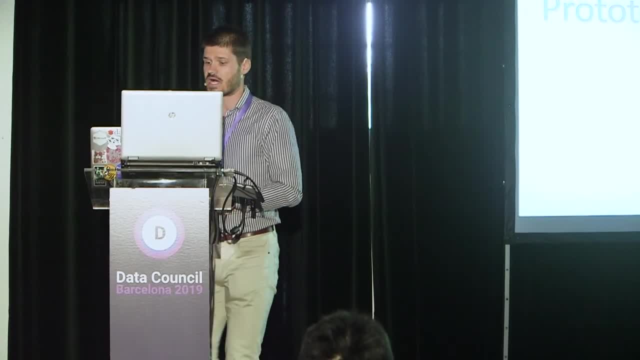 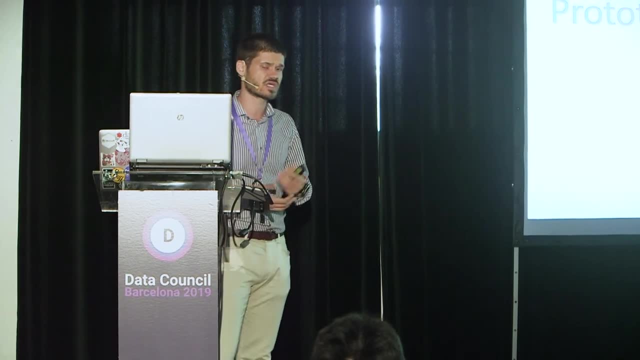 professional data scientist. you love code, I love code personally. sometimes it's worth to don't start always with code, and for that I'm referring when you have a small business coming to you with a small project. you just want to validate it, just give you some data and you want to see if that that probably is. 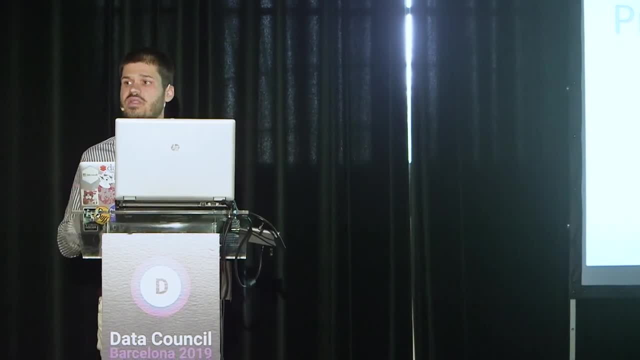 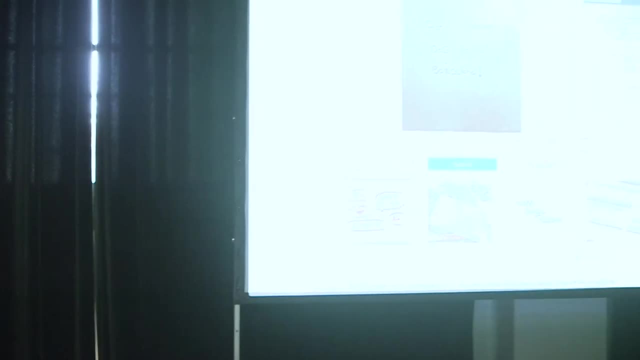 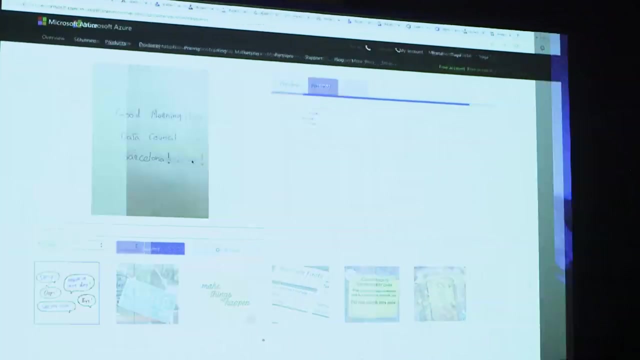 feasible or not. with the data science approach, sometimes it's easy to look at graphical interfaces, so what I'm going to show you, to you, is a possibility, if my screen allows me. okay, interesting, I have one screen there and a different one here. see if I can fix it. 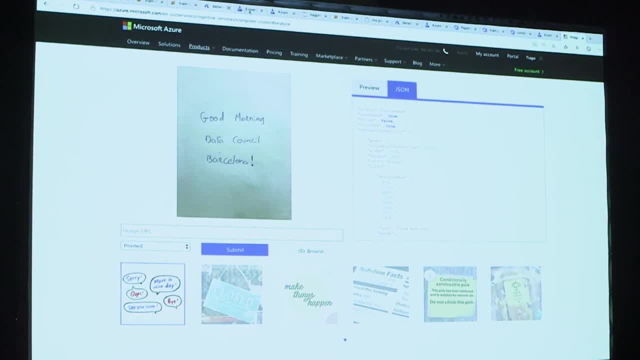 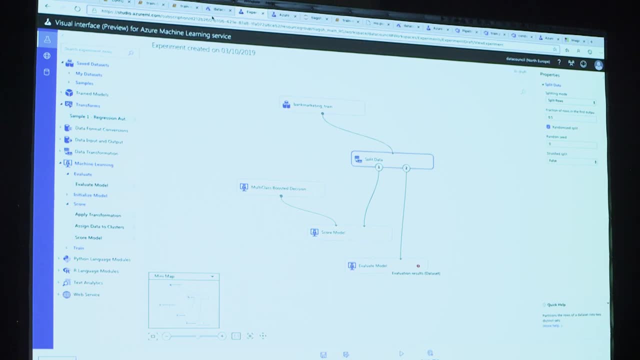 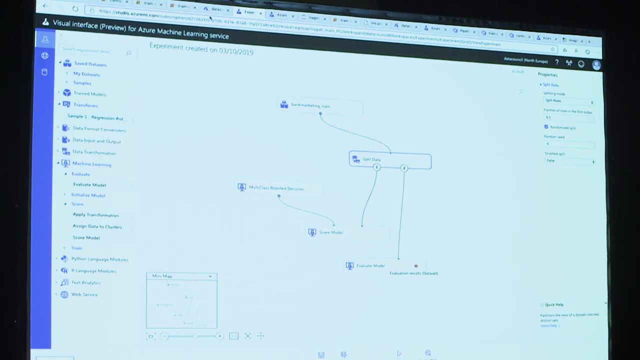 out of full screen. so one idea here will be to use a graphical interface to quickly mock up a data science project. it is also very effective for non-professional data scientists, typically citizen data scientists, business data scientists, someone who really understands the business as understanding of a machine learning problem. so there's a graphical interface. 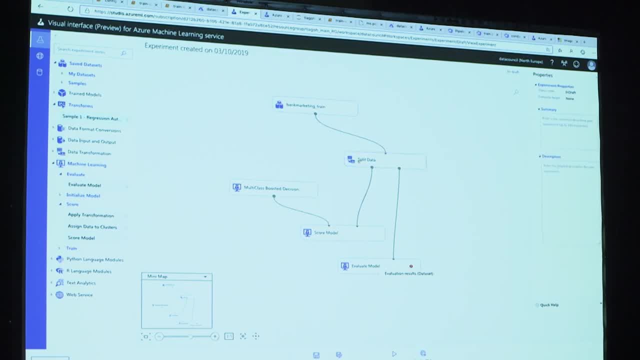 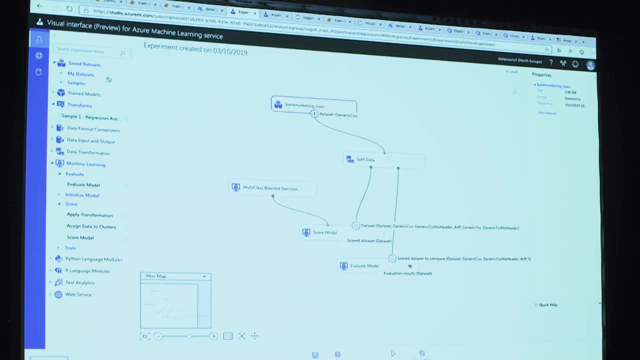 to do that. basically, as you can see, you just start to drag and drop boxes. this one, actually, it's already pretty done. I wanted to show you from scratch, but we are short on time. so basically, I'm importing a data set. in this case I have some simple data just imported here. I connect it to a split data to split my. 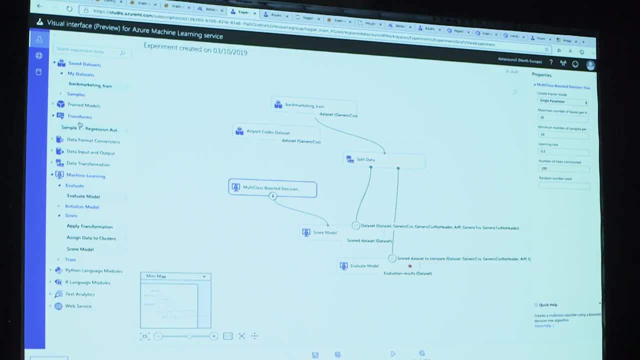 training and test data set. I'm picking one of the many available algorithms there and I'm going to show you how to do that. so I'm going to show you how to do that. as you can see, there is four: classification, closing, integration. I just pick one of them. of course, I can fine-tune some of the parameters then. 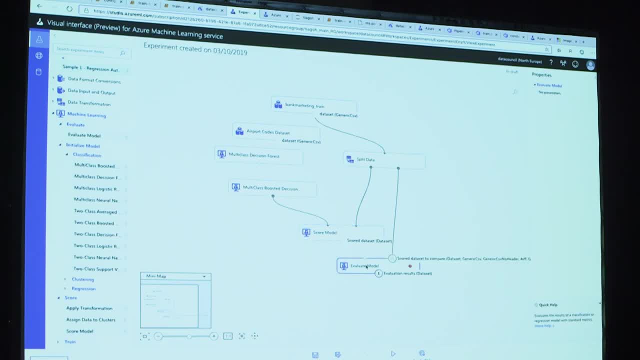 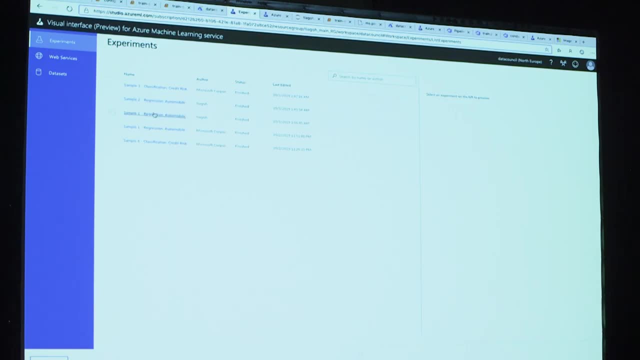 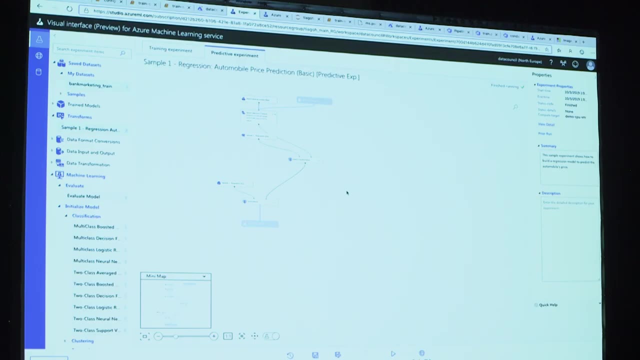 I'm scoring it, I'm getting the result, I'm getting the test set and evaluating the model. okay, to prove to you that this works, let me just go to the experiment that has been run already. when you run, basically specify what kind of compute you want to have behind the 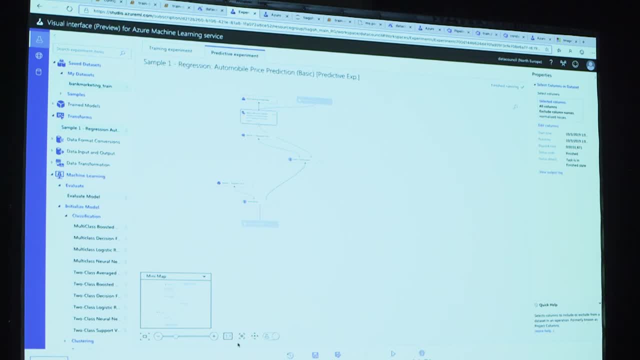 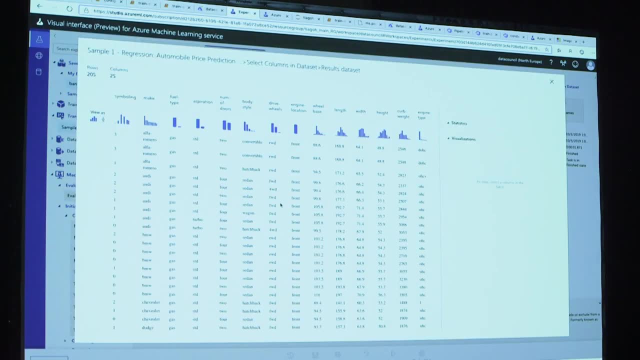 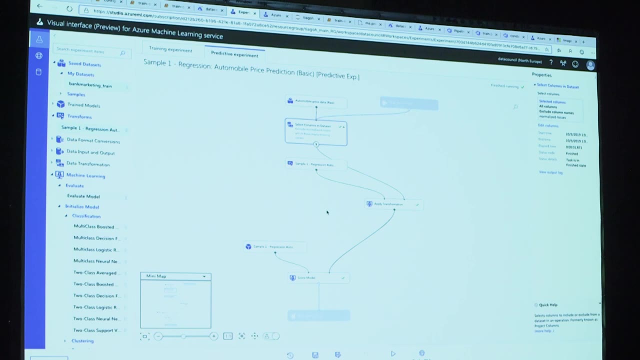 scenes, depending on how complex is the problem. and once is there, basically you just can. you can come here and see. first, look at the data sets. It's actually quite useful. once more. you've got the business data set, just want to look at it with some statistics. you get it out of the box and you run your model and then in. 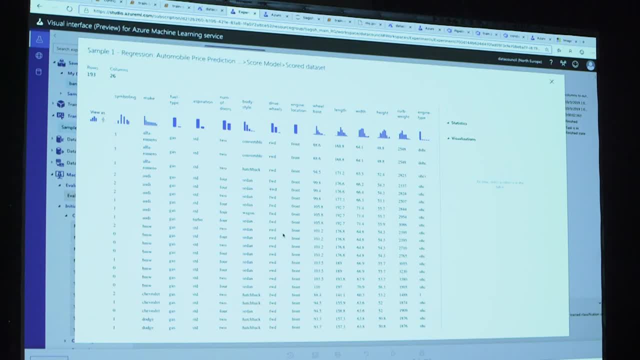 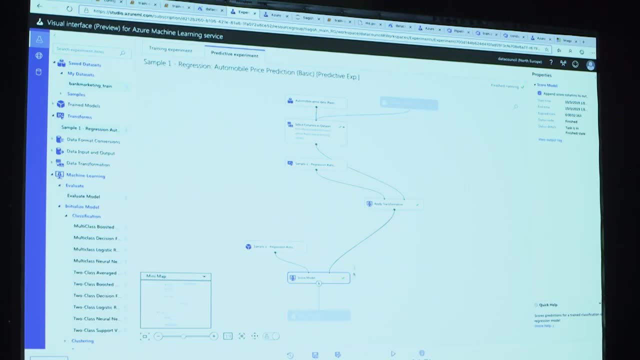 this case I just want to visualize the results of the scoring with my score labels. another very interesting thing here that you can do after testing your training, your model: you can click on deploy web service and literally with a few clicks- I won't be doing it now because I've done it before you're going to. 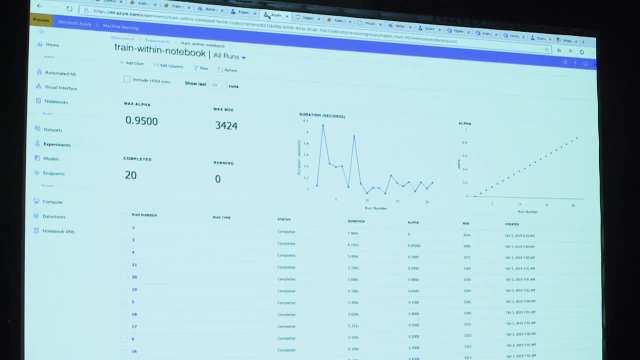 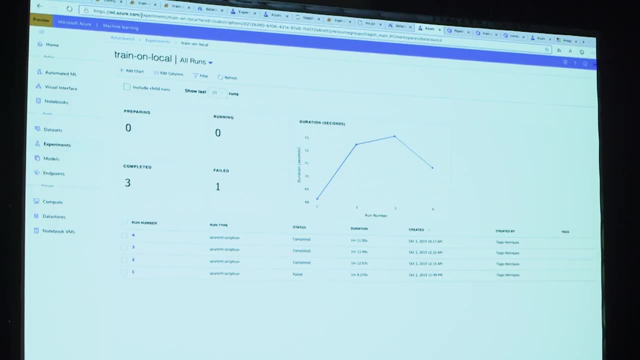 deploy your model as a predictive web service. Let me show you that I've done that just before to save some time, So I have endpoints. It means it was deployed from that studio I showed you before And, as you can see, there is a scoring. 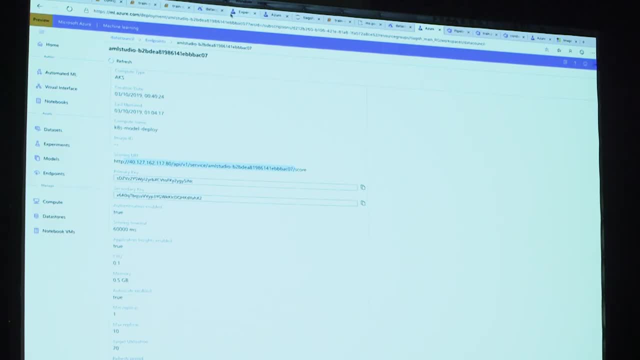 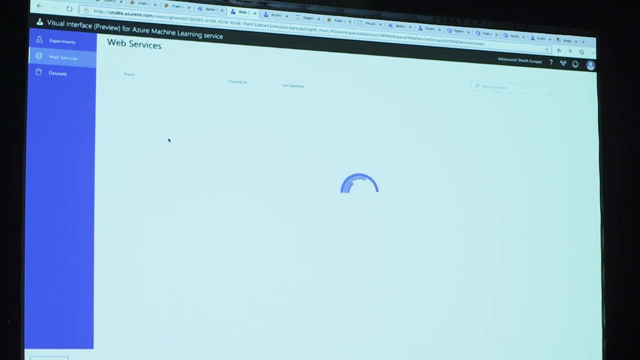 URI which I can connect to and make predictions. If I actually go back here- sorry, if I go back to web services. that's exactly what I wanted to show you before, So our connection is not helping me, so bear with me. 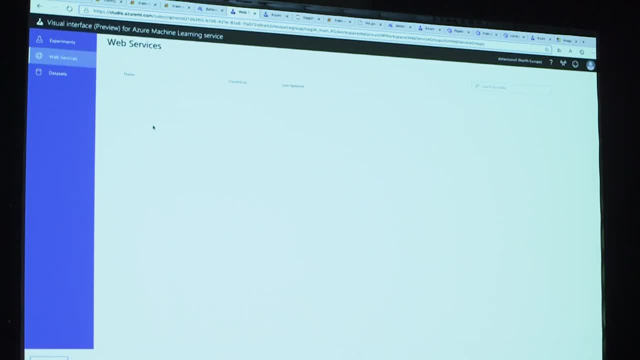 This is my deployed model I've shown you before. It's basically to predict the value of a car based on a set of inputs like the age of the car, how many kilometers, what was the initial price. So this is the deployed web service. It's deployed as a container, because that's. 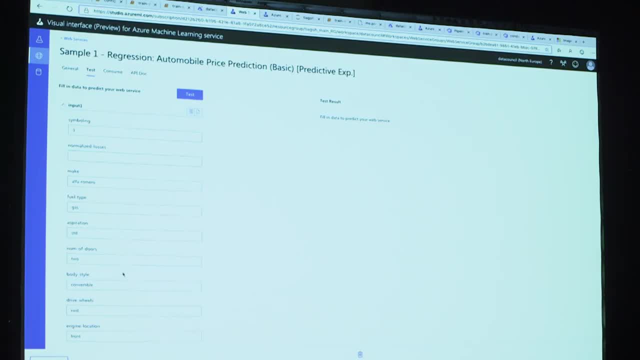 the industry trend these days. So these are the variables I'm sending to the predictive model and now I'm just sending those ones connecting to the endpoint and getting a result. And the result of the prediction in this case is the value of the car. 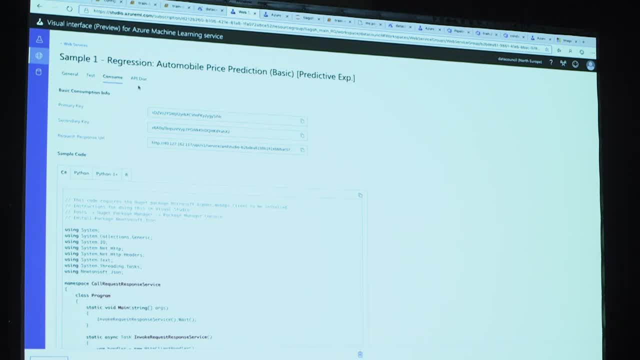 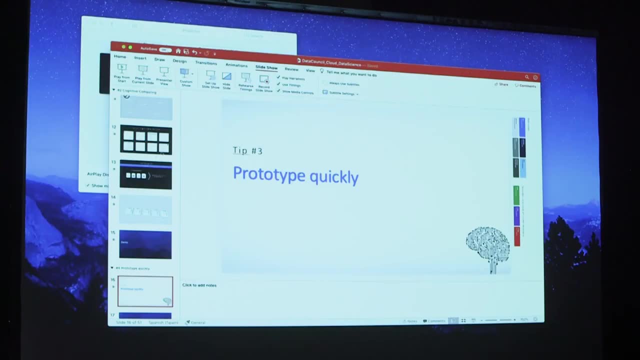 It gives you also out of the box, some code samples to connect by yourself or, if you really want to connect at low level, it has also the restful API specification. So you have seen within, just in this case, very little minutes, because we don't have much time. 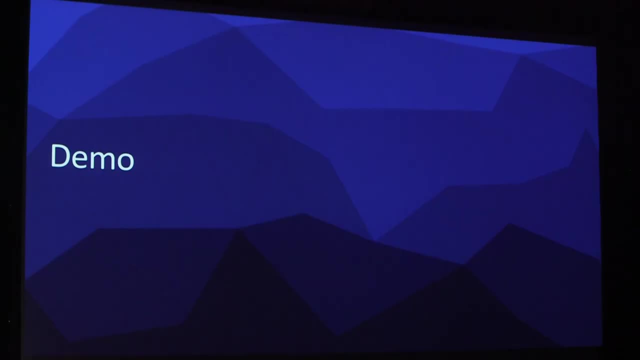 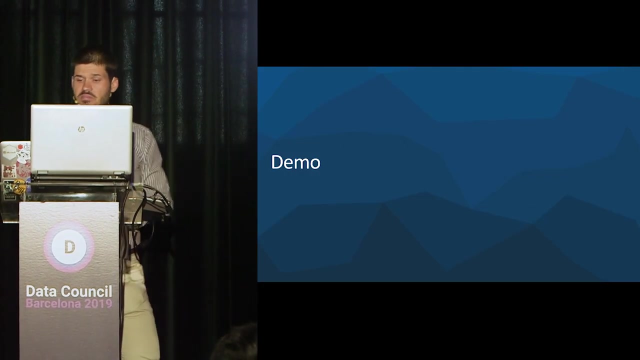 but how can you leverage a graphical interface to build predictive models? I forgot to mention that you can also bring your own code, so R and Python can be in the middle of your floaters, So you can still code and basically auto deploy that as a model. 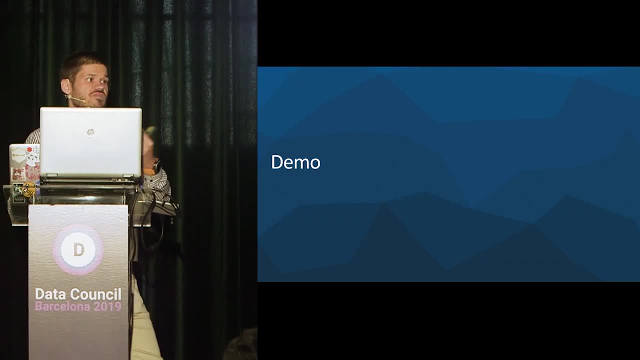 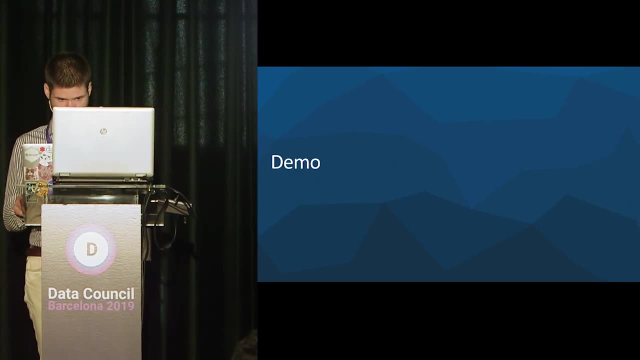 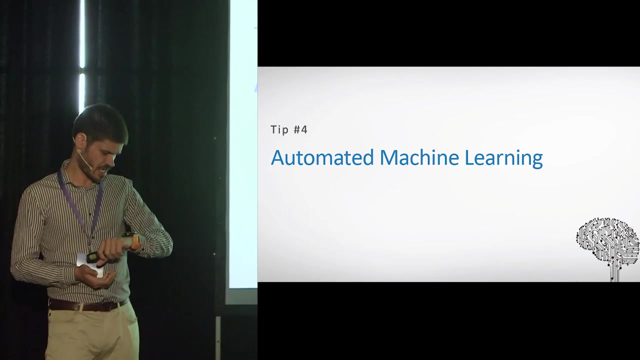 So I think it's a very valid way to prototype quickly and sometimes even to take your experiments further and faster. Okay, Next thing. next tip I wanted to show you is about leveraging automated machine learning- Anyone using it on your day-to-day practice. 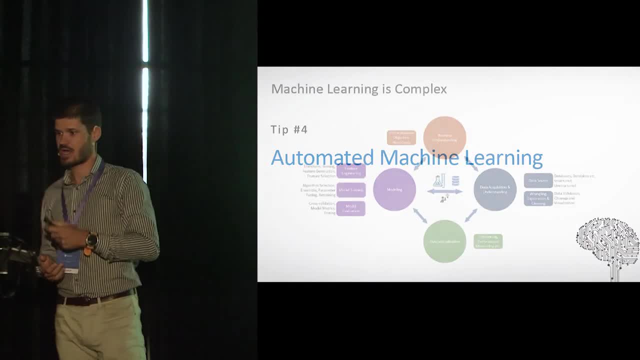 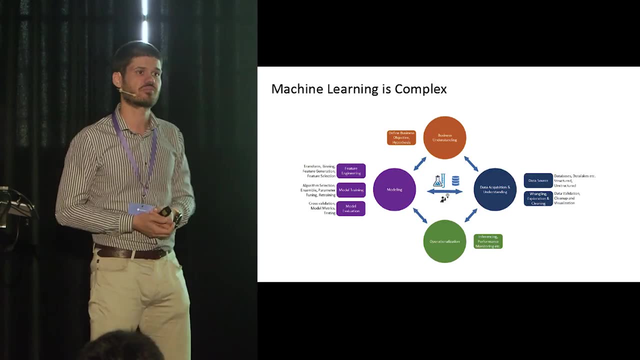 Is that already One person? Okay, That's a good sign. So automated machine learning is a very important thing. So machine learning basically tries to make your life as a data scientist a little bit easier. As you know, when you start doing a predictive model, there's a lot of time behind the scenes. 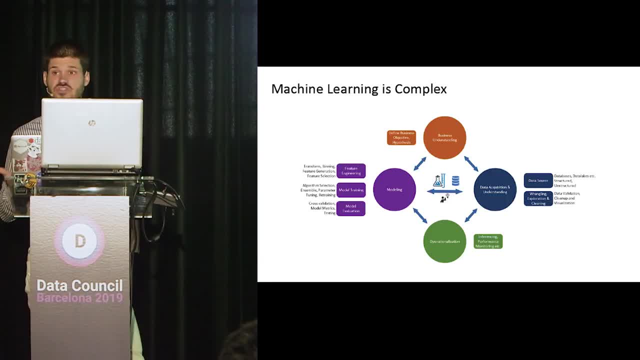 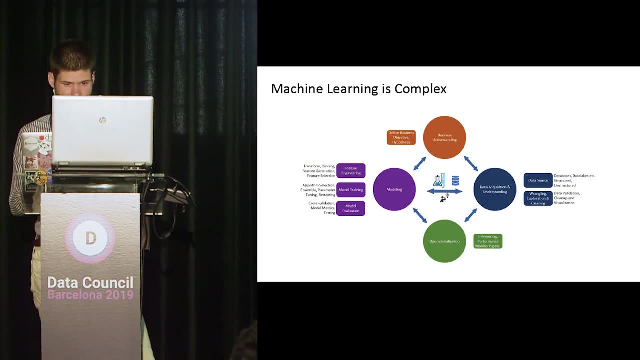 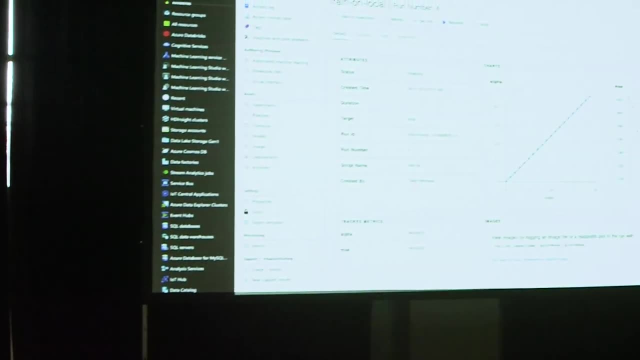 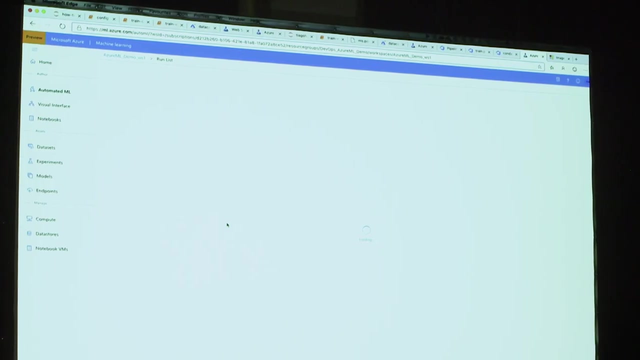 of trying different algorithms, different parameters and fine-tune them. That can be really, really time-consuming. Let me skip a few animations and show you how it works in our graphical interface. The idea behind the scenes is, of course, as a data scientist, of course you know better. 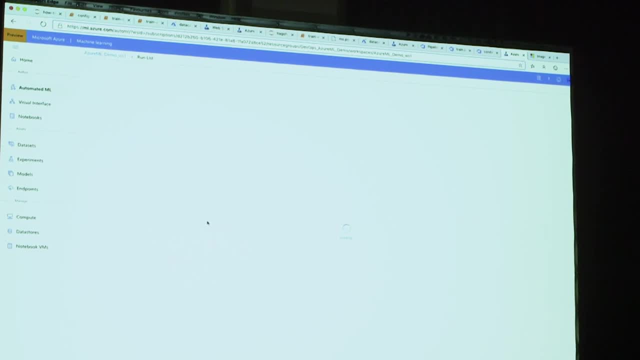 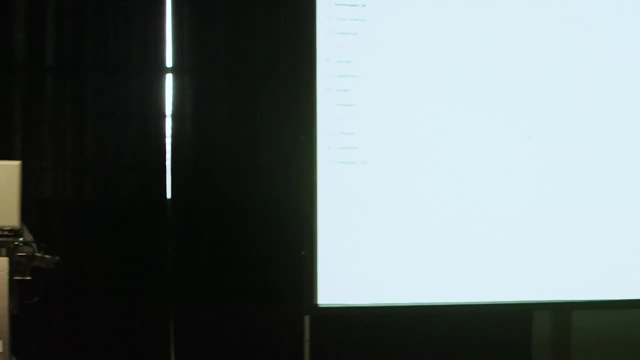 than anyone how to build models, the best models. but it can kind of automate part of your process, Basically testing a lot of different algorithms, test them in parallel and fine-tune all the parameters, which I think can save you a lot of time and by the end of the day after 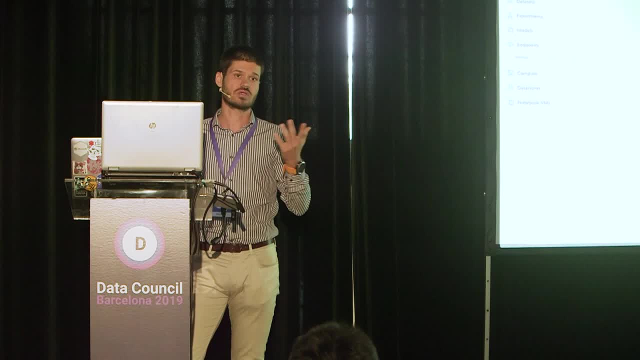 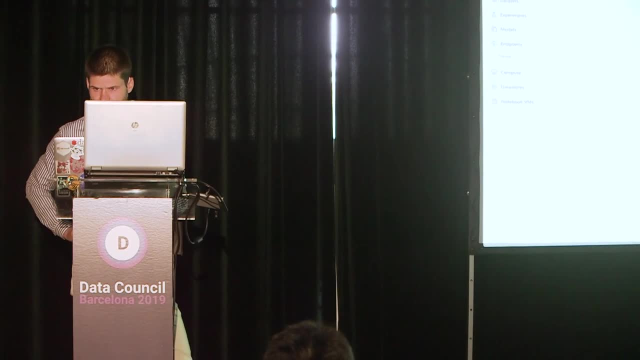 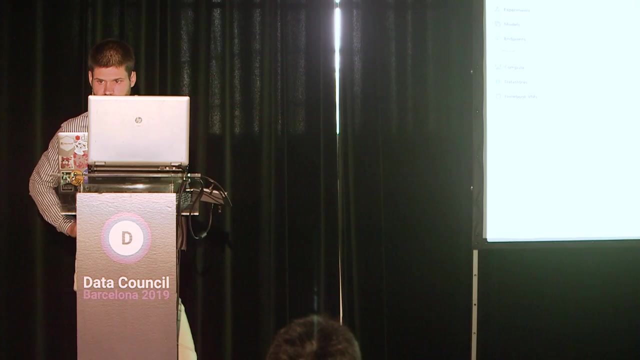 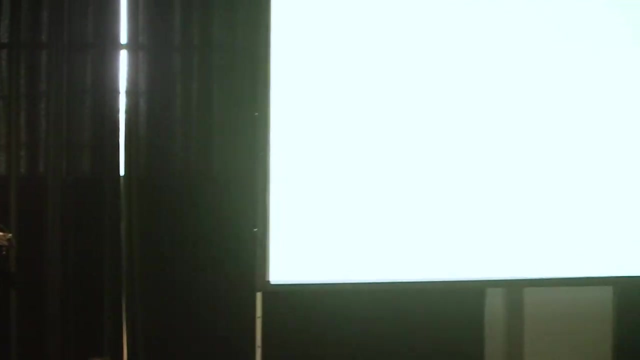 you've run these kind of experiments, you can still retrieve the model and see what are the variables that are more impactful and, based on that, still keep carrying on your job. I think the connection is not really helping me a lot. I prefer to show you the real thing than just the animation. 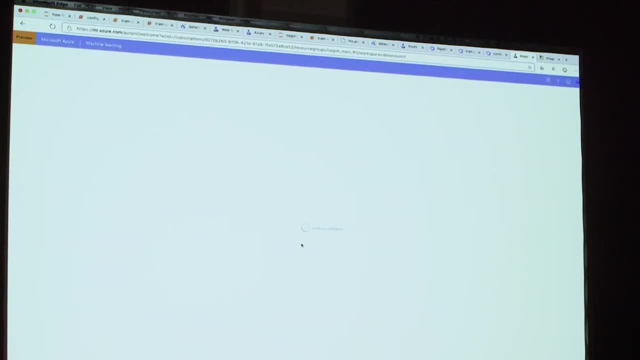 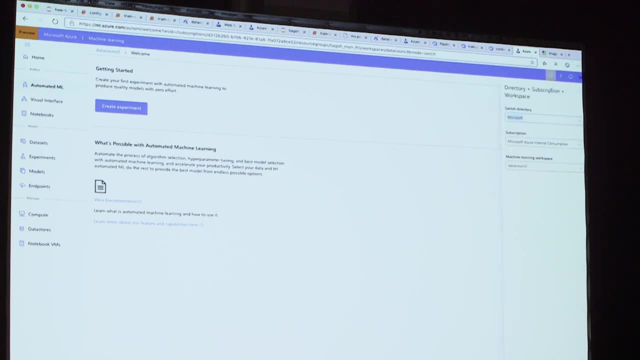 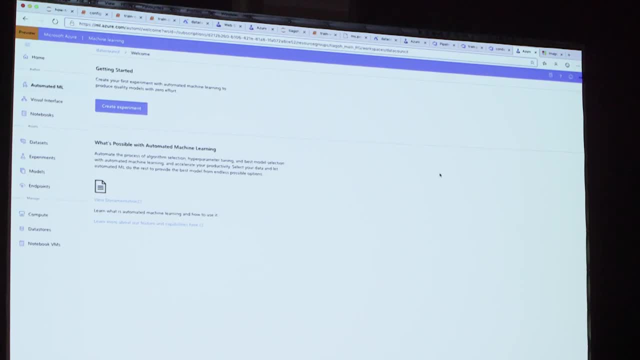 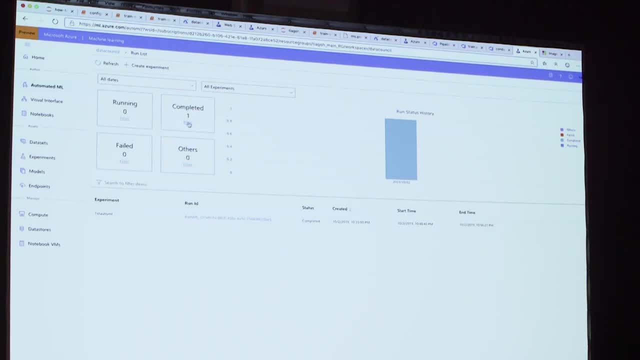 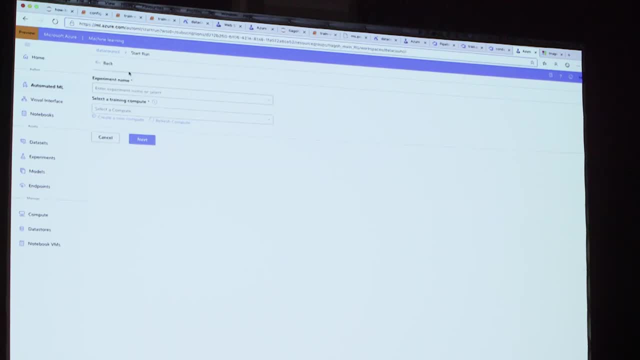 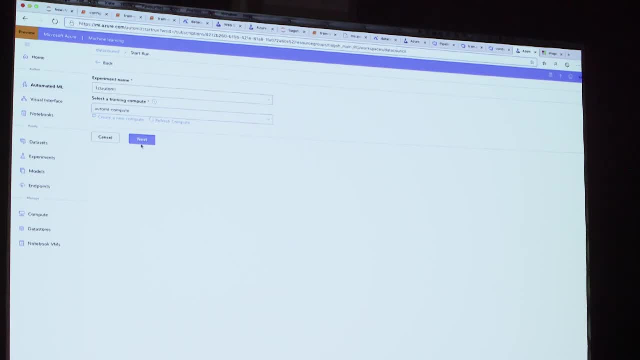 Let's give it a try Now. I'm just specifying the name of the experiment and what is the compute behind the scenes. I'm loading a data set- This case is a banking data set, a public one- which basically is about trying to detect. 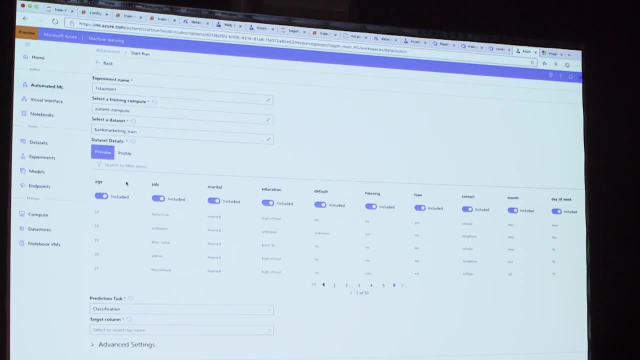 if a specific loan or offer I want to make to the customer will take it or not. You can see the variables: age, job, lot of data them. It can very easily say, for example: don't include I don't know day of the week. 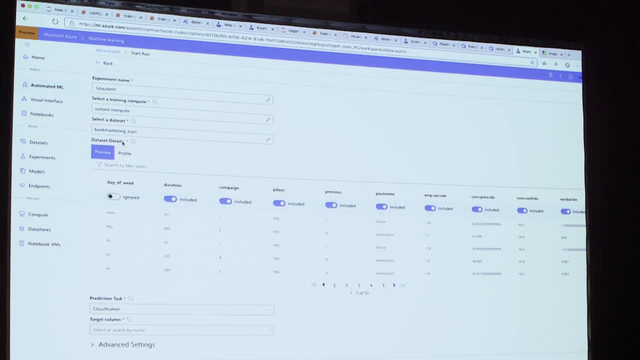 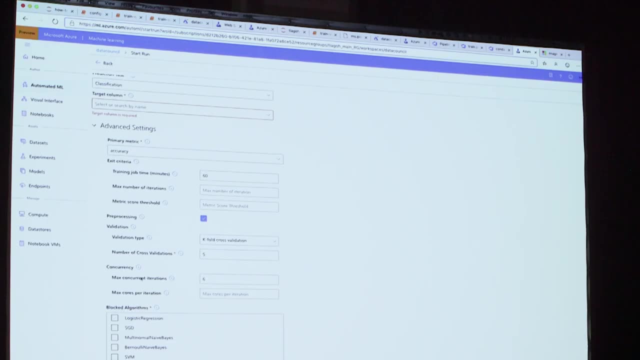 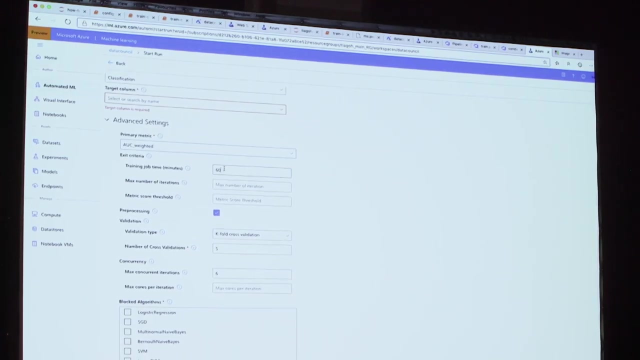 might not be included. You can look at the profile of the data per variable And then where the automated machine learning happens is here. Basically, I'm saying what metric I want to track on. In this case I'll take AUC weighted. How long I want this to be. 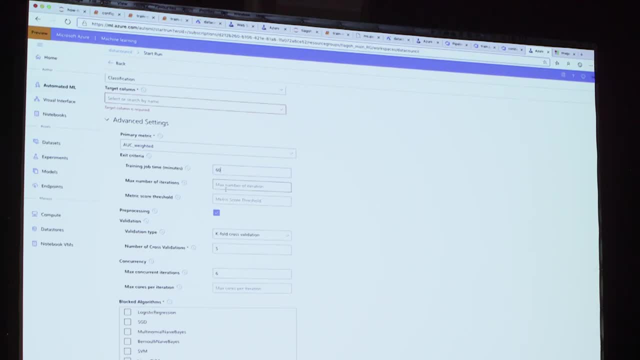 running, because it can be running for a lot of time and also, of course, the cost of its running is impacted to you, Or the max of interactions you want there. What kind of validation you want to make: Number of cross validations, The concurrency, which is interesting. 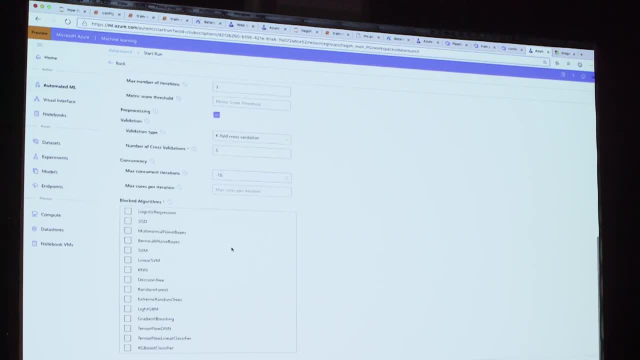 You can start to parallelize things and save some time And basically a lot of algorithms that you want to try. or if there's something that you specifically don't want to test it, you basically say: I don't want to use those two SVM and linear SVM. Okay, After that. 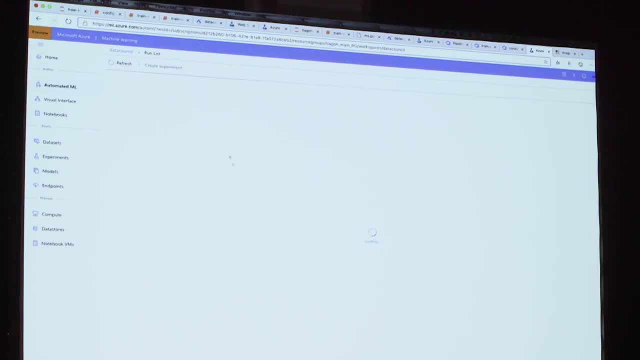 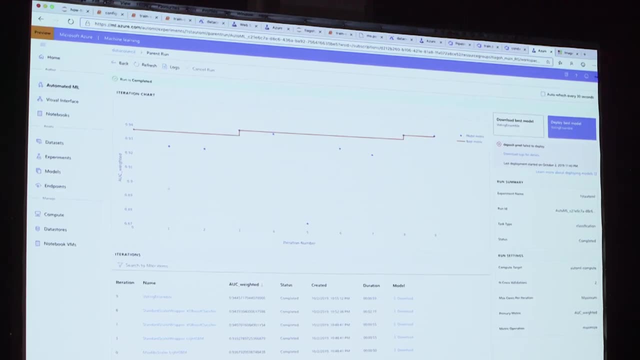 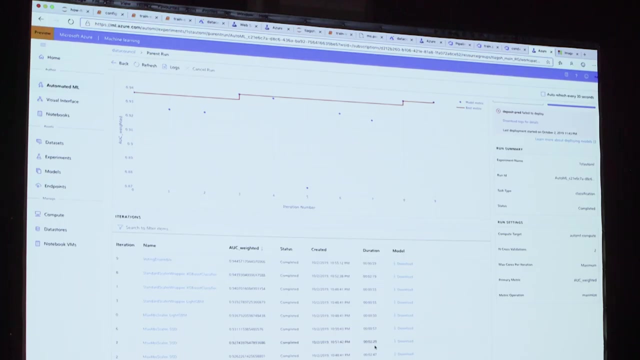 it submits, It of course needs a few minutes to get started And once it's run, you can see. As you can see, these are iterations over time And this is the metric I'm tracking AUC, So I can see here, for each algorithm first, how long it took to train on each of. 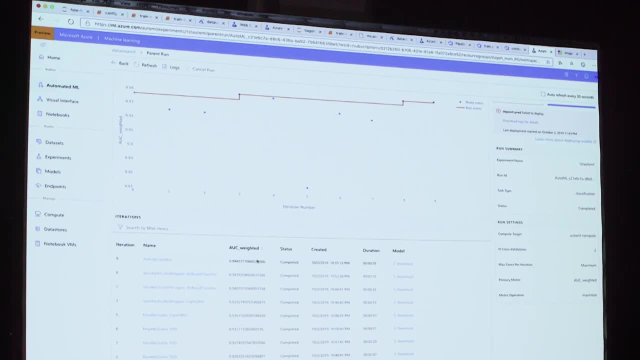 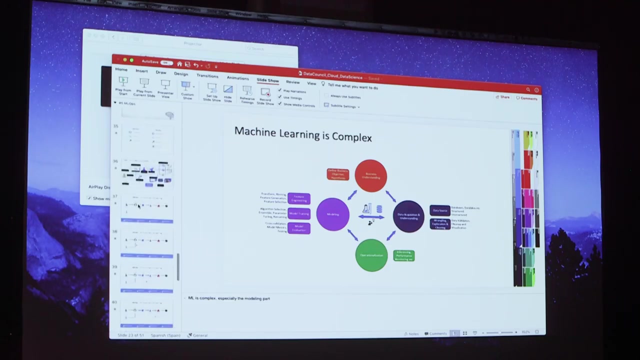 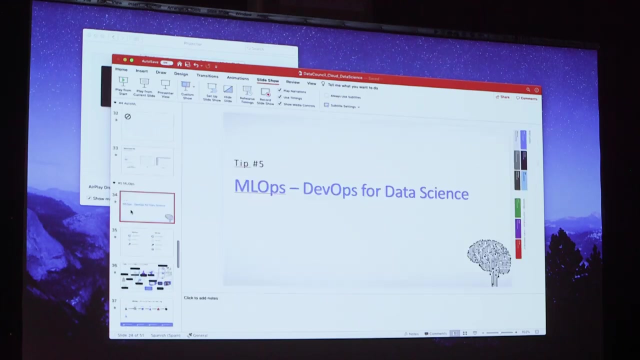 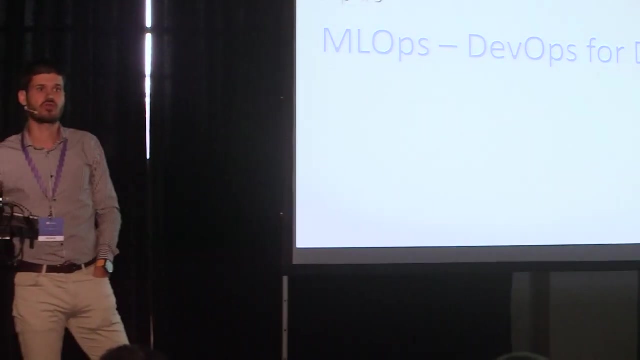 them And then, in this case, I want to see which one performed better, which was the voting ensemble, which was actually, I think, the last one there on top right. Okay, Very interesting to automate part of your machine learning processes. Okay, So my last tip might be the one that might be a bit more outside of what you've. 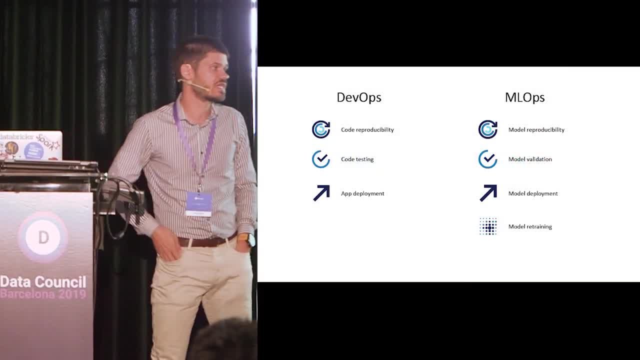 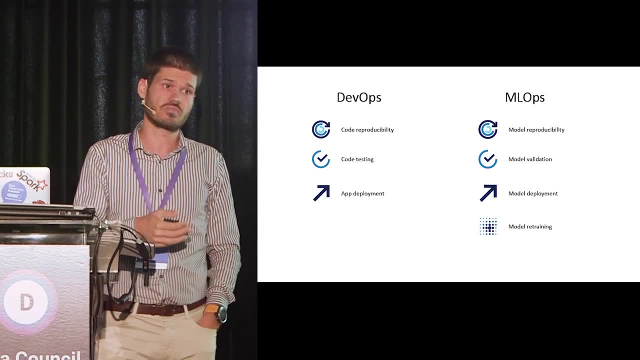 seen on data science projects- If not, I'll be very happy- Which is really about helping you to build kind of, if you want to call it, a machine learning factory, Basically being able to chip more machine learning models into production, Make sure that they are tracked. 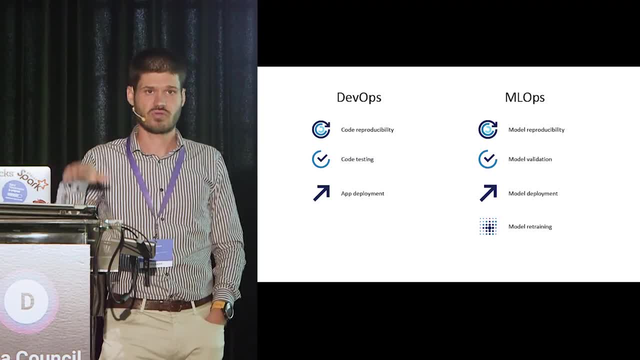 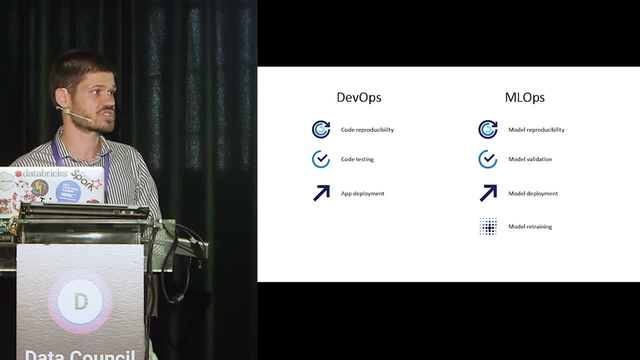 and that you can detect, Okay, That they are decaying performance over time And you can automatically retrain them. That's kind of the idea. Of course, for that it requires, I think, a big change in processes and, of course, the tools behind them. The idea here is to embrace the concept of DevOps. 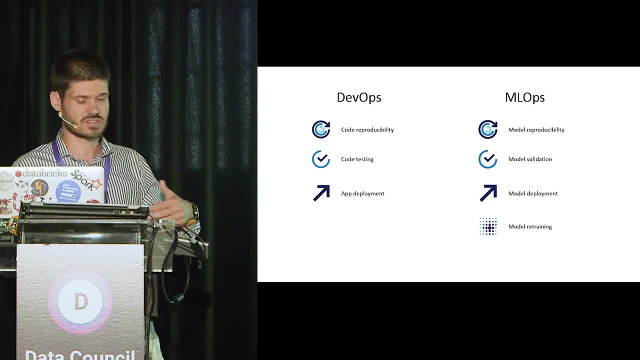 Everyone talks about DevOps these days, Really about the iterative: experiment fast, experiment quick, fail fast and have a complete feedback loop. That's the idea with general software development. Reality is in machine learning world. it's slightly more complicated than deploying a. 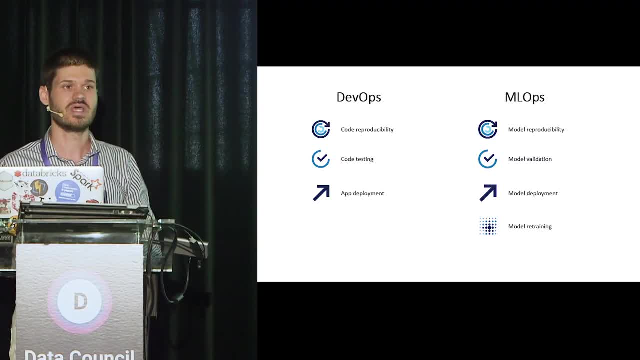 web application because of the data and the models and the performance, And that we know that over time, models will decay accuracy when they are deployed. Okay, So there's a few things that I think are important if you want to embrace this concept of machine. 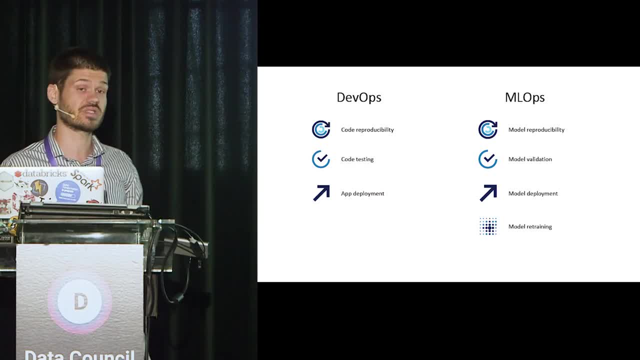 learning operations, which is basically, of course, reproducibility. That's why I started with the experimenting, Then validation. Of course, automation, machine learning might help you there, but that's an optional step. Then, of course, how do I deploy models and 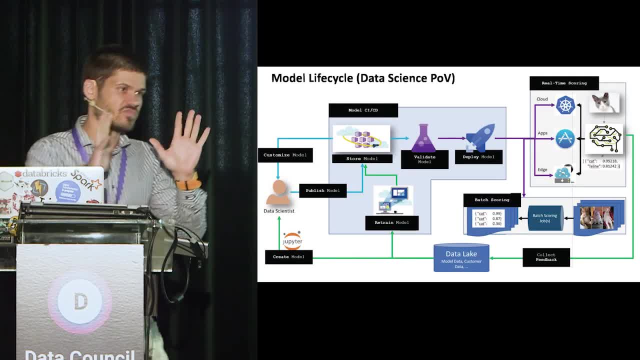 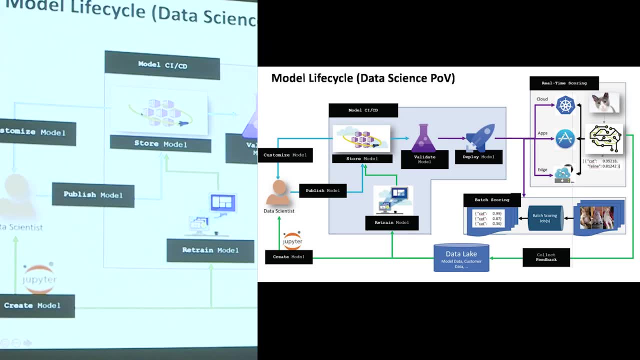 how do I retrain them? So, from a very generic point of view, the idea is you have a web application, you have data scientists, like most of you guys, training your models. You should be able to have a central place where you have what we call a continuous integration, continuous deployment. 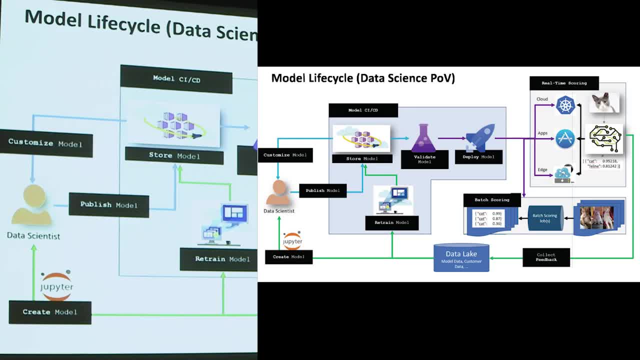 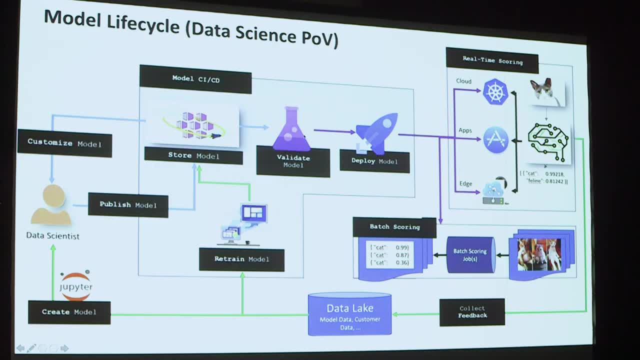 pipeline, which means that your code is basically, every time you change your code, you make a comment to say, behind the scenes, I want to automatically, for example, run some tests on my model and deploy my model into pre-production or test environments. I think it's really interesting. 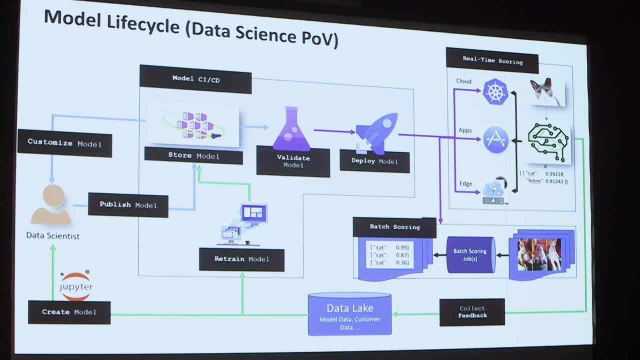 because of course, it brings extra engineering skills to data scientists, but also give you the capability to really implement it. So that's the idea behind the web application: You can really deploy your models, test them and, potentially, if you have some applications, 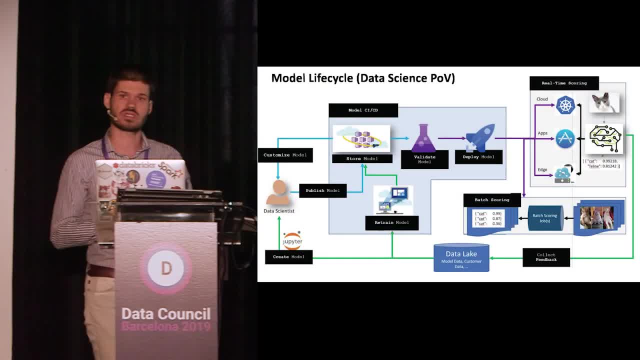 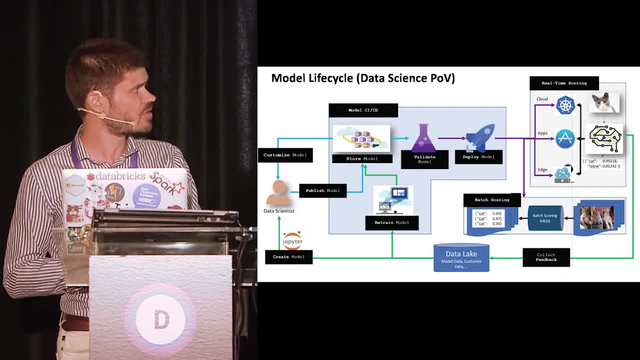 or even dashboards that you want to connect to your particular models and see how it looks like and show it to the business. I think it's really a good way. So that's the main idea. Secondly, over time the models will decay in performance, So the idea is that we collect. 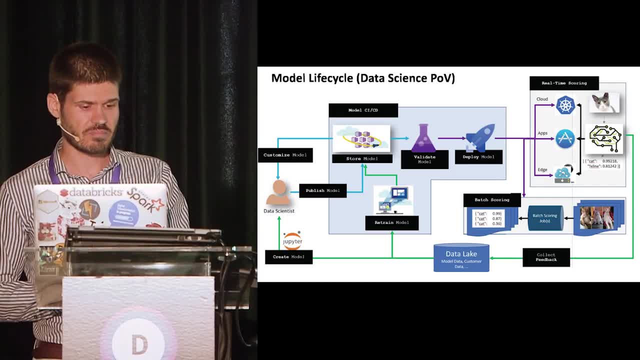 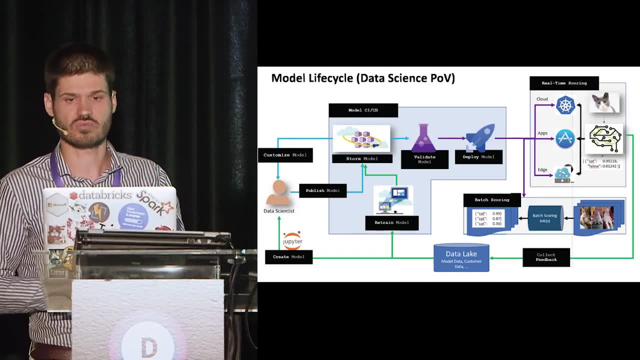 the metrics of the models, we centralize them in some place and basically I will retrain the model, hopefully to improve it, or if it doesn't improve, at least I should be able to detect that and in worse, in extreme cases, take it out of production. 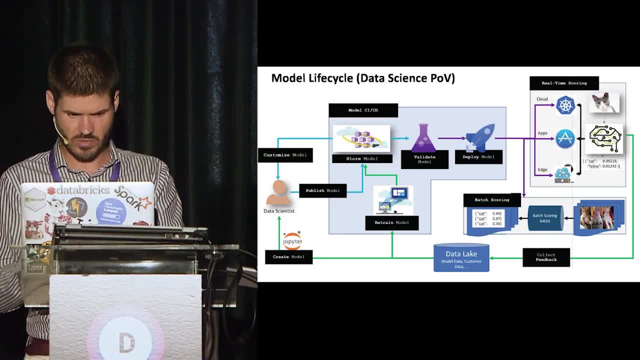 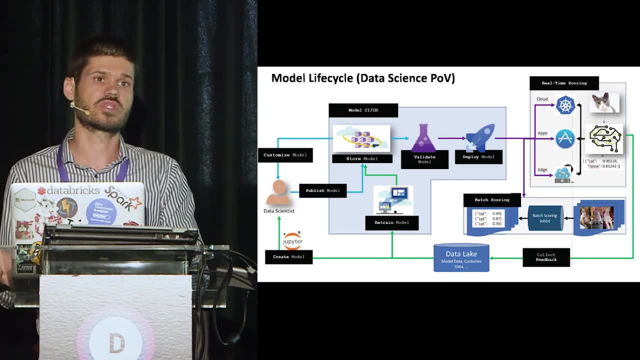 So, without going further, I'll just show you a small demo. There's some slides about each and every step, but let me just show you a demo. In this case, we use a specific tool for DevOps with the idea to use for machine learning processes. So here I have a very 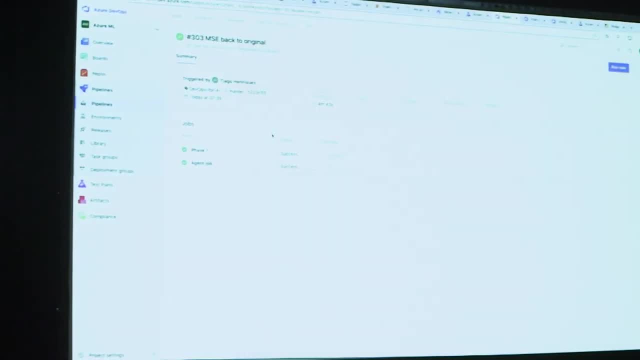 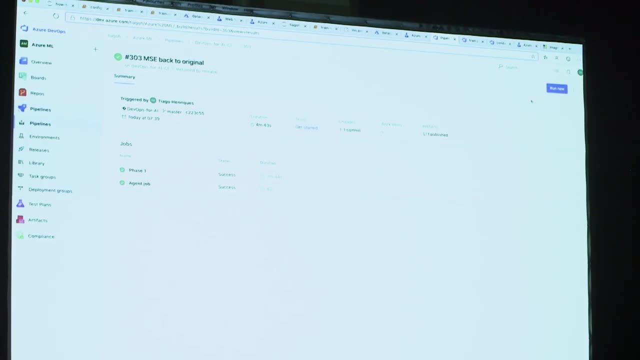 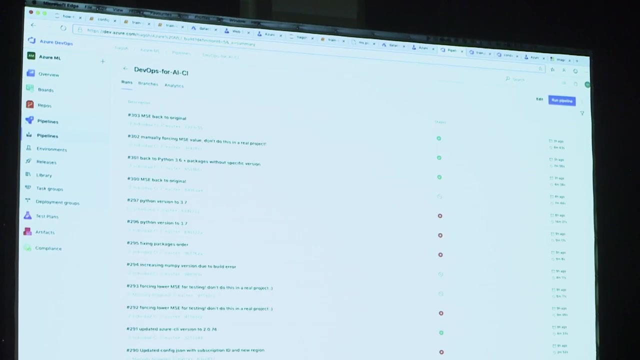 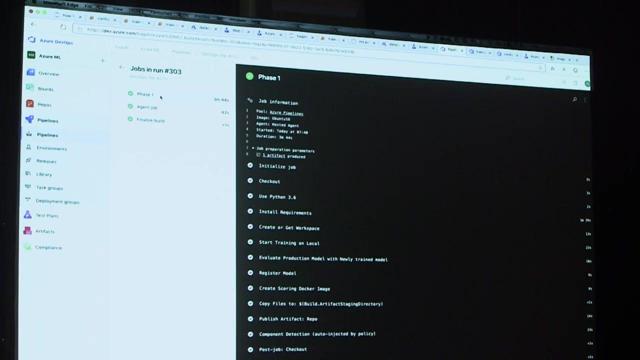 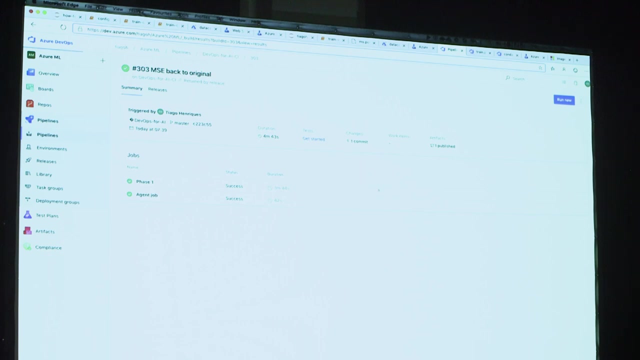 simple pipeline that I've defined before: machine learning pipeline for continuous integration. Let me show you what it looks like. So what I'm doing here is defining a few steps. One of them is I'm just saying I want to use Python, and then the most relevant one for data science is: I have a few scripts. 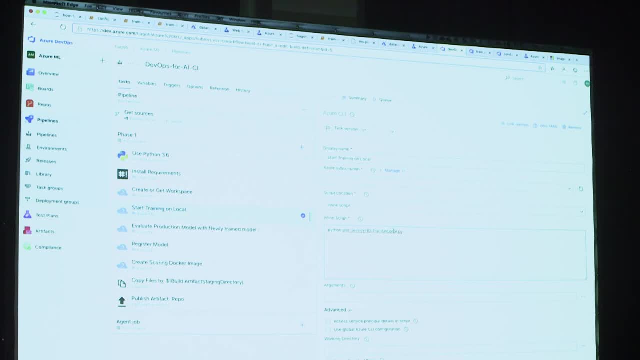 in Python you can see which one is training. that's very similar to what I showed you in the beginning. Then I have another script to say: I want to evaluate my model. Once my model is evaluated, I will register that with a central register for model. 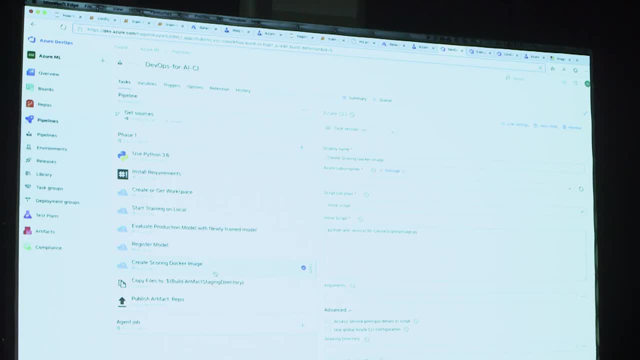 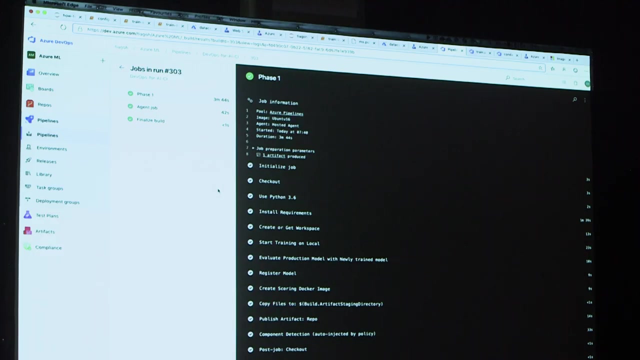 so I can track all my models into production and then generate a container to potentially deploy that. I've run that before and basically takes, in this case I think, three or four minutes. Let's pick a successful one. Remember this is every time I save my code. 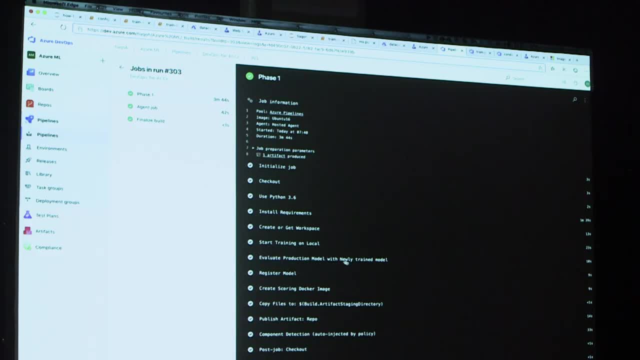 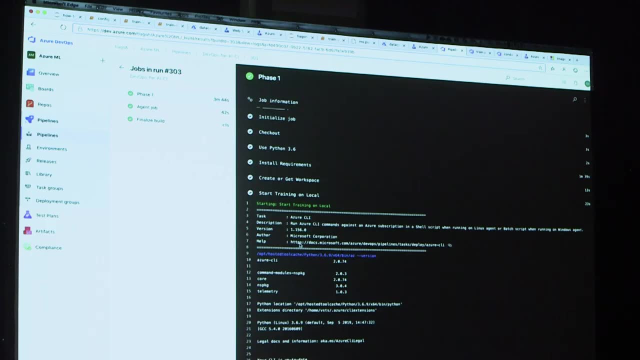 or I commit something. this happens behind the scenes, so it doesn't affect my job as a data scientist. but, as you can see, for every step, starting, let's say, maybe, with start training on local- local is some machine, remotely in this case. 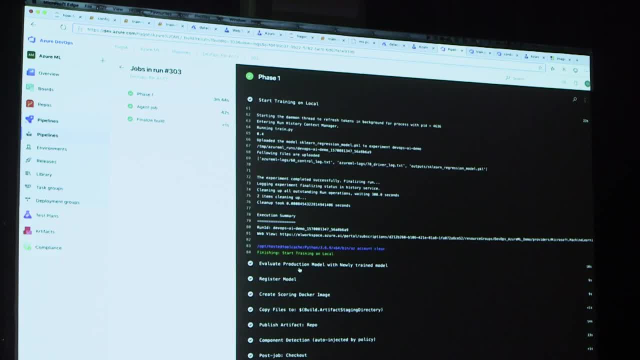 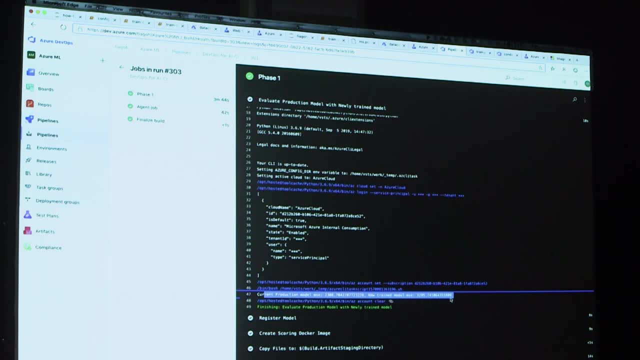 then, well, before it was installing packages, then I'm running evaluate the model. just takes 10 seconds registering the model and in this case, the interesting part, maybe for you here, is this line: It says that the model I have currently in production 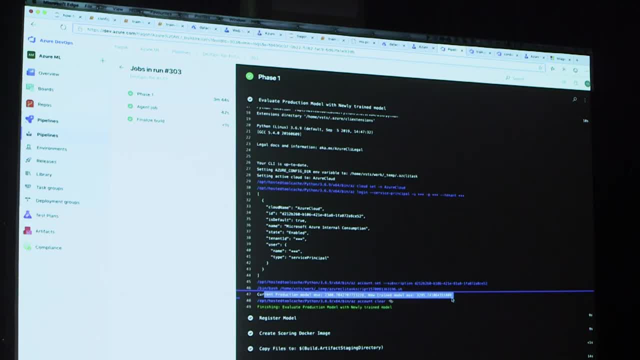 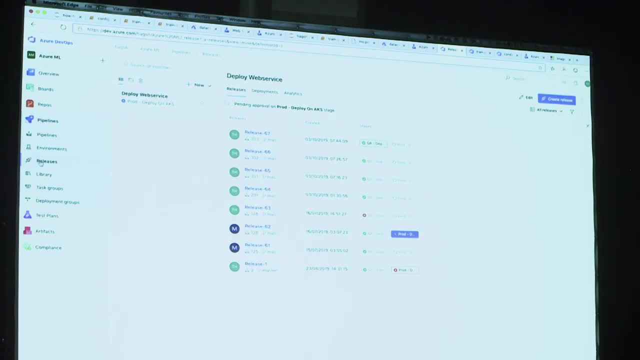 has this amount of MSE and a new one has that one. so, based on that, it has some logic to say: do I take it into production or do I just keep it okay? And finally, when the build- because this was just automated- build of your codes. 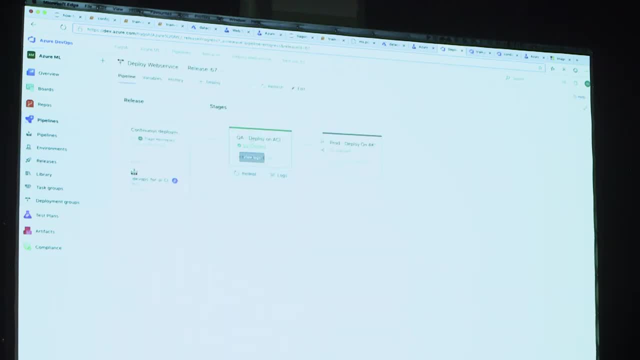 is done, I might have a way to release that into production. In this case, I've deployed this as a single container Behind the scenes. it took, I think, five minutes. so once more, it's an API exposed. I can consume it. 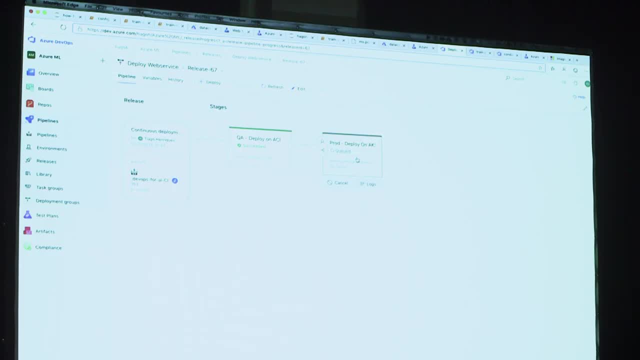 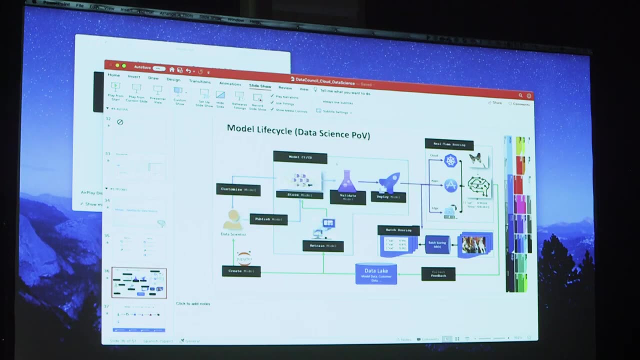 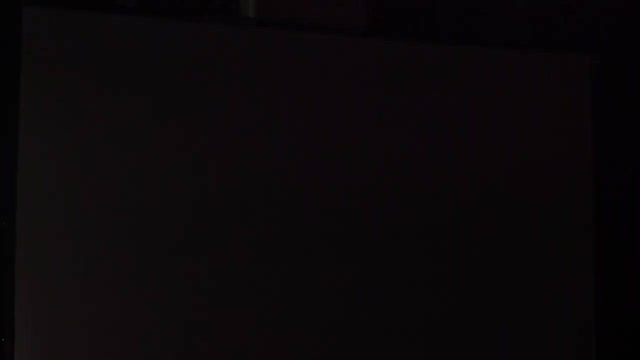 and if I want to take it into production, I could make a trigger and of course, production things are very sensitive, so it might need a human to go there and approve that. That's kind of the idea. Okay, Okay, just two. one extra minute. 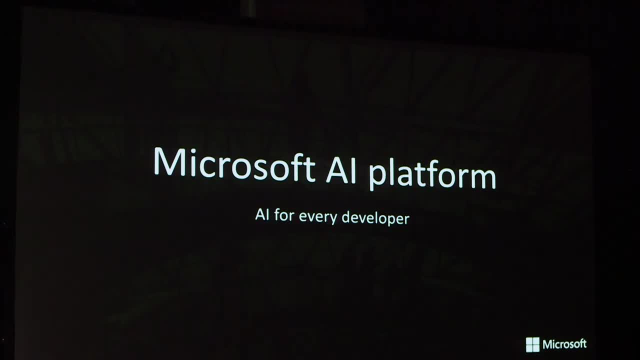 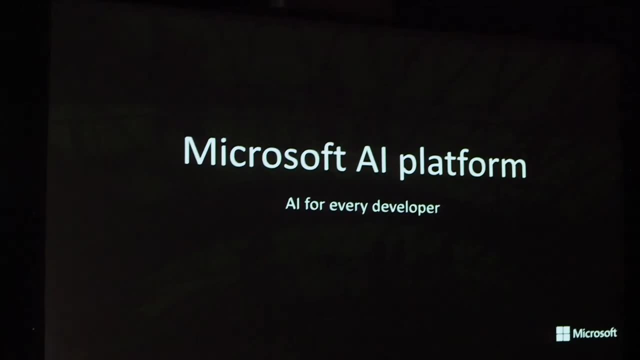 I know we went a bit quick on a lot of different concepts, but basically the idea is that, as Microsoft, we've been doing, of course, machine learning for more than 25 years. We've been investing very hard and a lot. 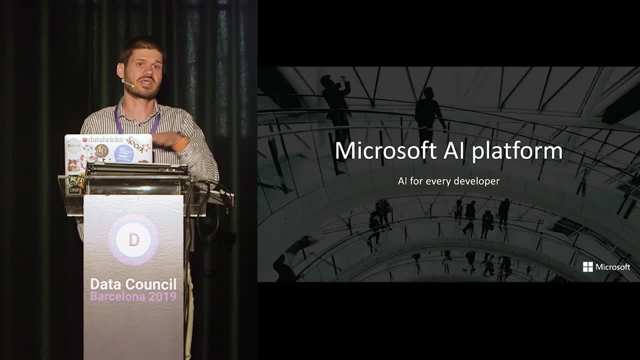 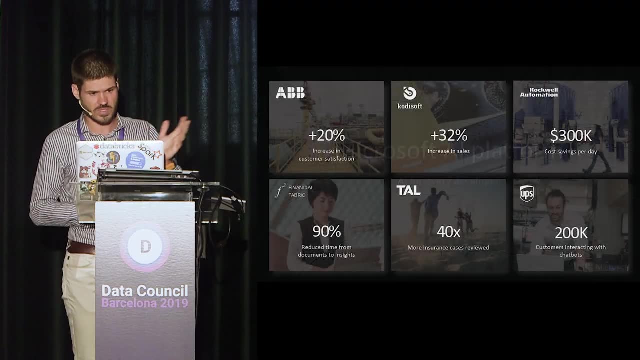 on bringing artificial intelligence and sophisticated machine learning tools for any kind of profile, from professional data scientists, citizen data scientists, application developers, the ones just to build some AI. That's the capabilities of our platform, My experience, like I told you, with big companies. 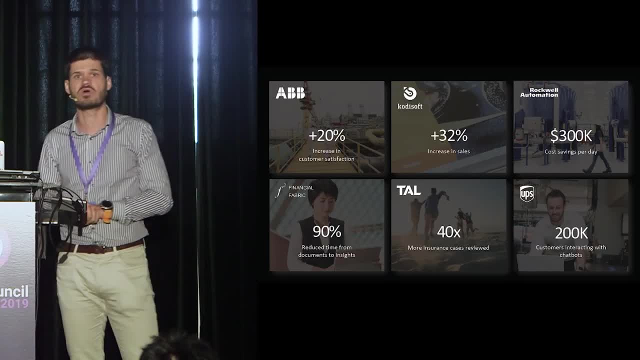 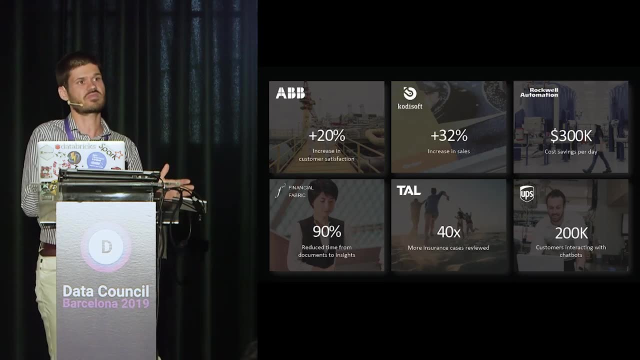 and you see names of big companies and the business impact they had with adopting some of these processes and tools. I think it can be very big, especially when you think about scale: scale from data science perspective, but also scale from industrialization of your machine learning models. 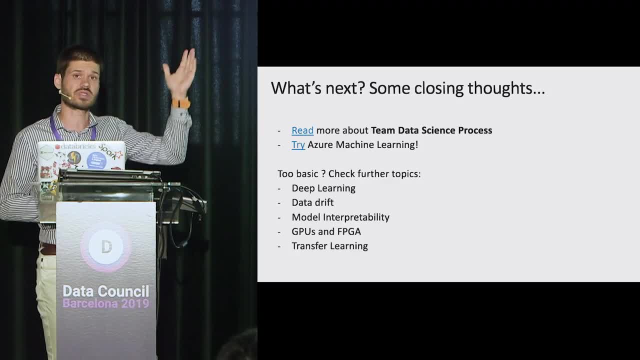 My closing thoughts and you're gonna have access to the slides- two things. One of them is really about the data science project. It's really similar. It's too crisp, but I think, more modern, If you want to try Azure machine learning. 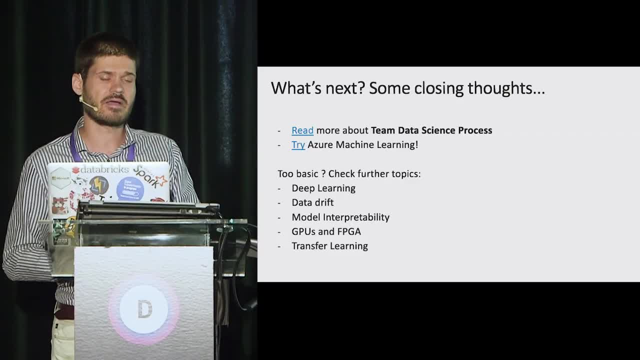 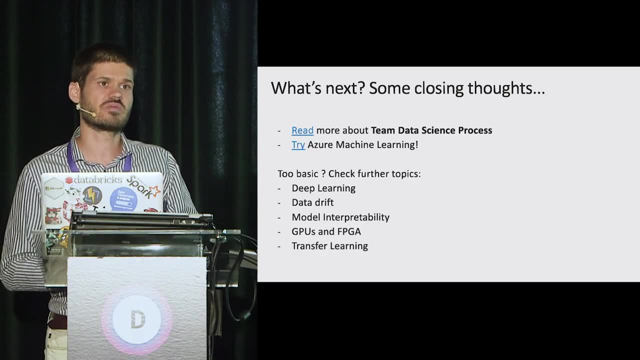 I think it's extremely interesting because of some of the features, And today we didn't go very deep, but there's a lot of other concepts that I think are worth to make your data science process even better. Particularly, one of them is detecting data drift. 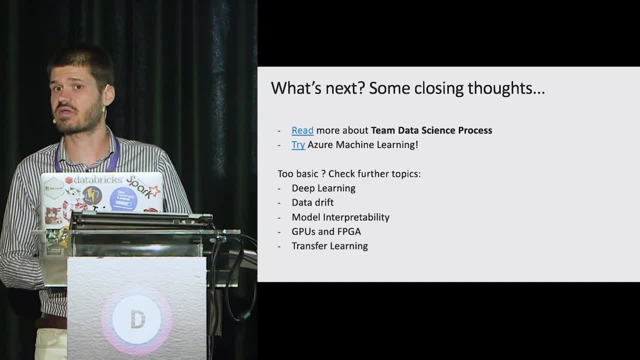 manually or automatically. when you have models into production, A big question I get very often from customers is: how do you interpret the models behind the scenes? So there's also capability to have modern interpretability and, of course, leverage the hardware. 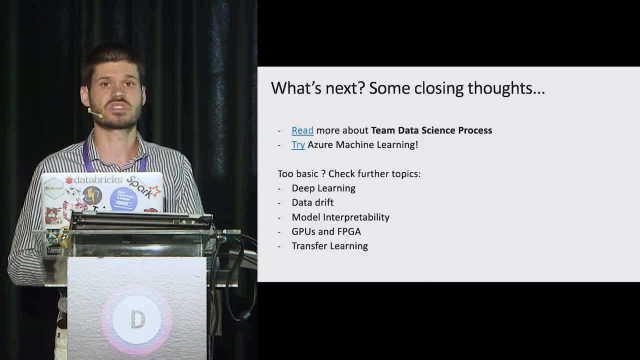 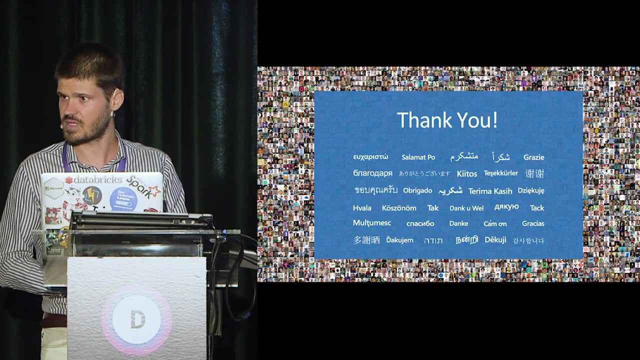 GPUs, FPGAs and so on. These are really cost-performance efficient when you have complex workloads such as deep learning. Okay, and with that, I think we are on top of the time. I appreciate your time. Feel free to ask any questions, now or later. 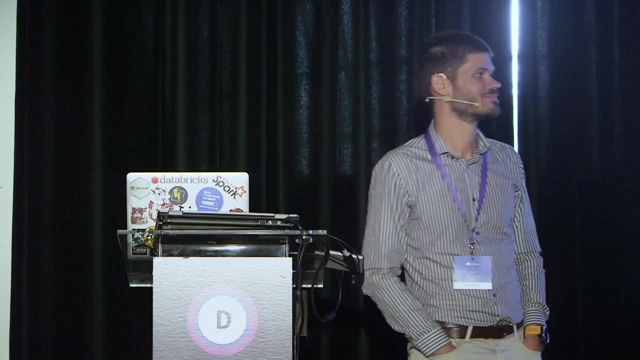 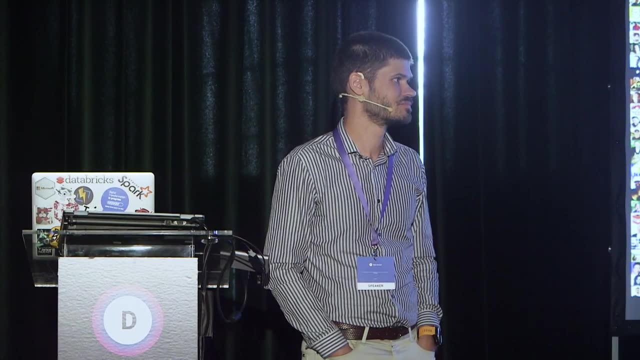 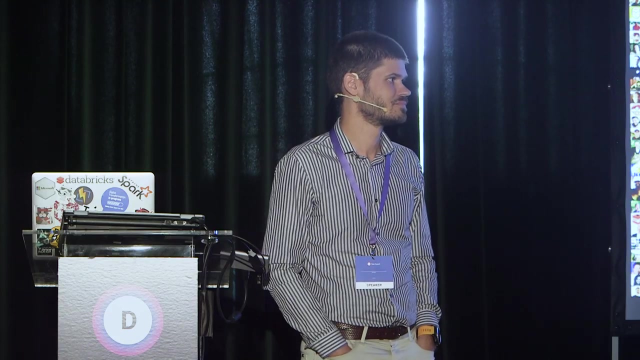 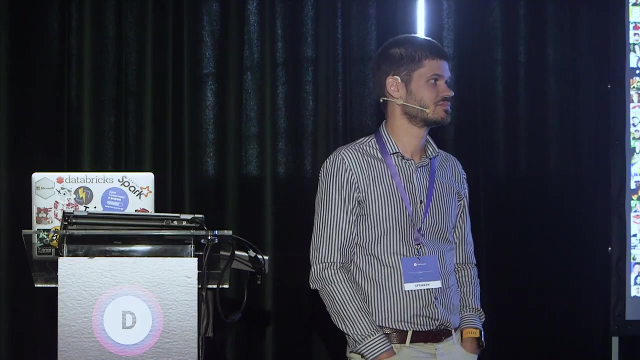 or reach out to me, Thank you. Thank you for your speech. How is your system, your UI interface, how is it suitable for using deep learning models such as TensorFlow, based on TensorFlow framework Sure? Is it possible to load some pre-trained models? 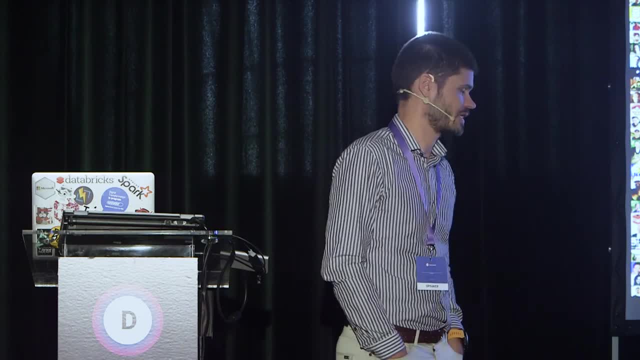 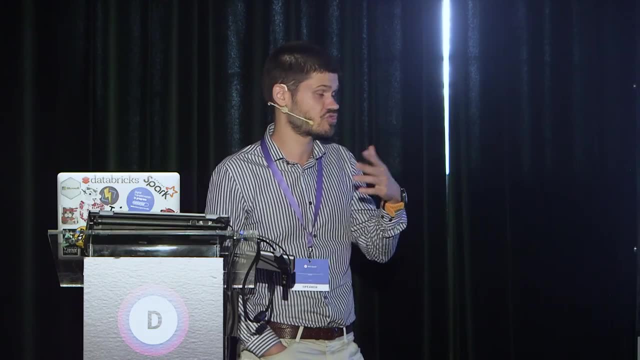 from Metafiles or something like that. Thank you. Yeah, good question. thank you, I didn't go too much into that detail. Today, the system you've seen, which is on Azure, it really tries to be a non-opinated system. 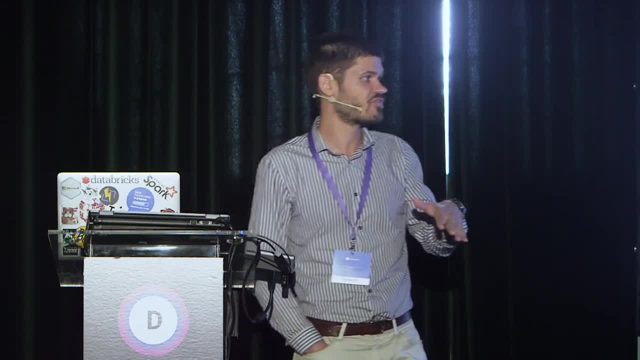 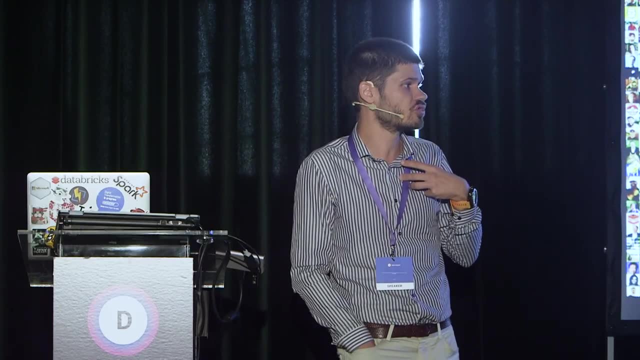 which means that we just want to let you leverage your favorite tools. By that I mean you can use any open source framework, including PyTorch, TensorFlow or any of them, So you still control completely your code the frameworks you want to run. 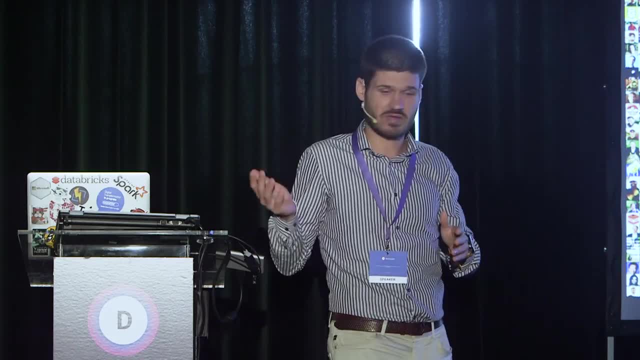 so it's completely compatible with that. On top of that, optionally, like you've seen, I was running a very simple training in a big VM. I could be running the same training in a GPU VM, of course, to improve my time. 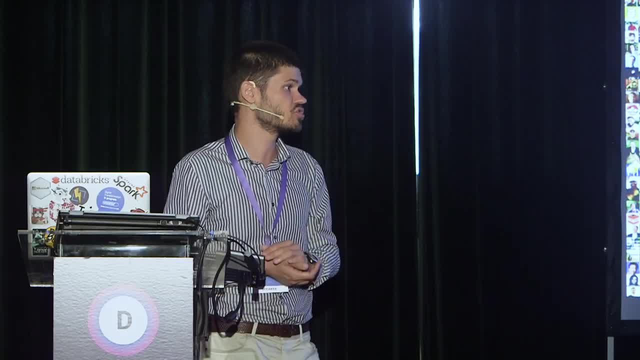 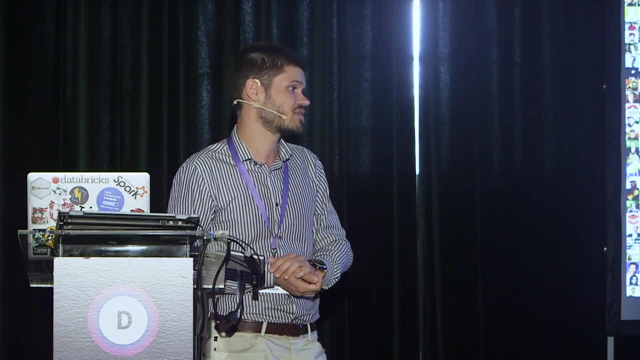 So the answer, yeah. bring in any framework and you have infrastructure like GPUs on demand, which is very interesting. You just use it for a few hours and you spin it down, which is a big cost-effective. I noticed that when you are running this. 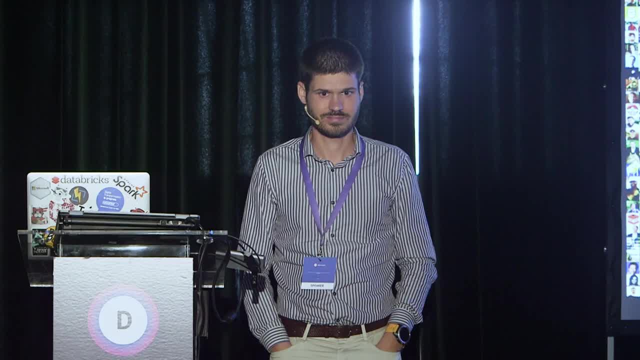 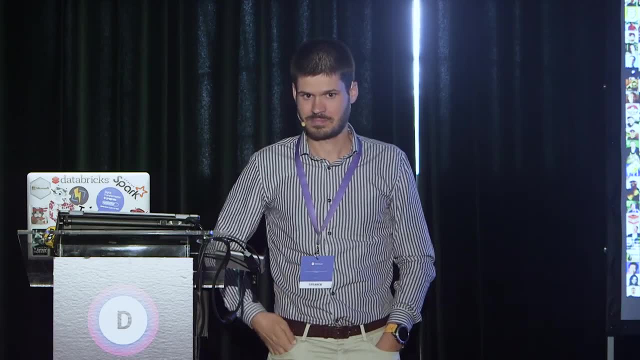 it keeps you constantly complete it. You constantly complete. there's no internet which slows down your process. So is it true that this Microsoft Azure will heavily depend on internet connection? So there's only one version, which is cloud version, right? 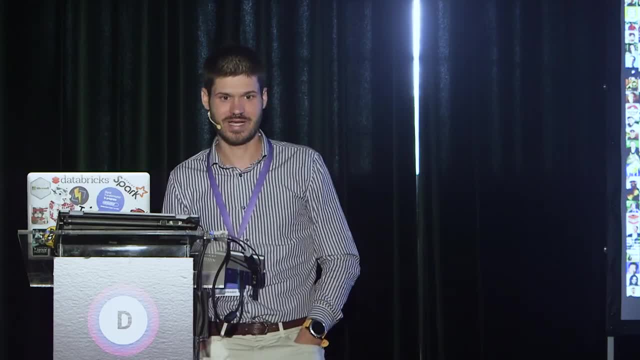 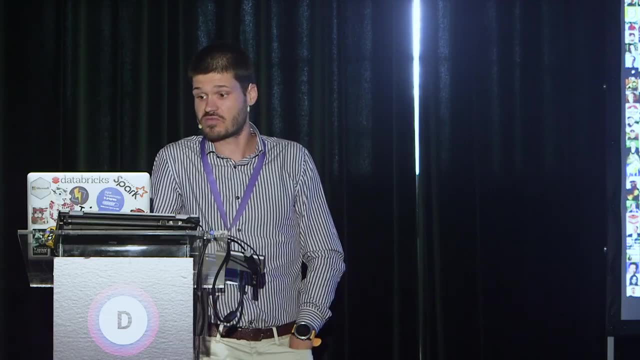 Yeah, so I think we need to have better internet connection for sure. When I test this at home or in my laptop in the office this morning, it works perfectly. So I think it's just if you have low latency, of course, you experiment that. 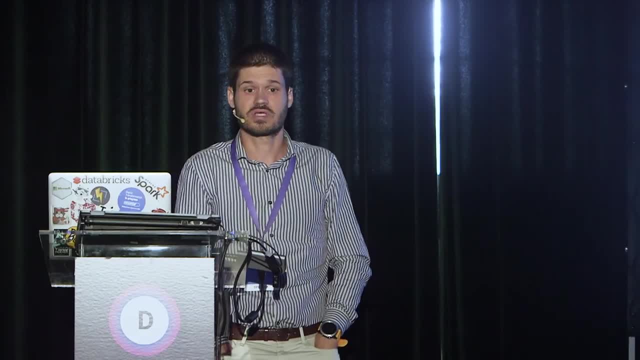 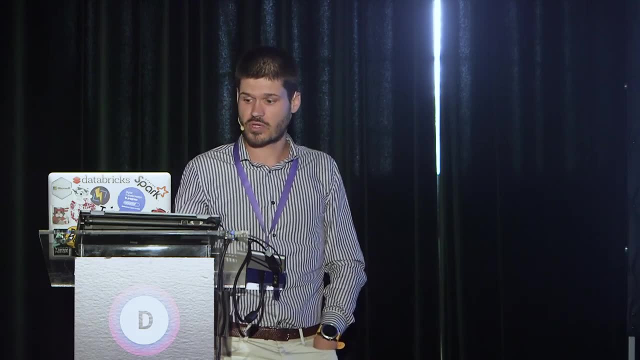 You're right, That's accessible through the public internet. Of course, that's the main idea with cloud computing in general, not just the machine learning capabilities. I showed you the example where you can start on your laptop, but to get all these capabilities. 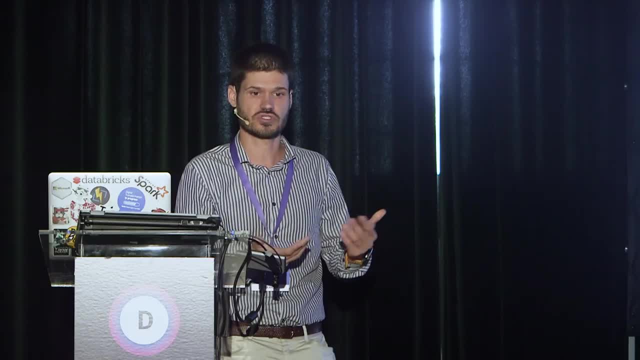 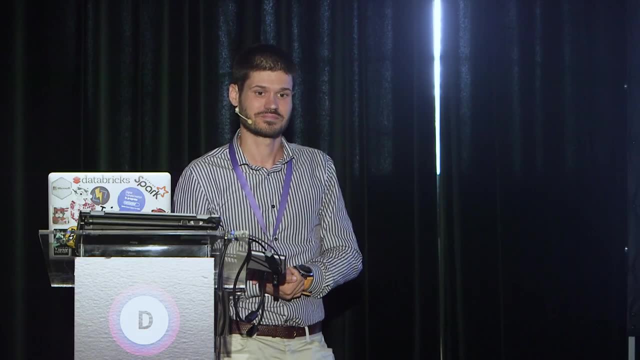 doing automated machine learning, CR experiments, leveraged GPUs. of course you need to have some connection to get to the endpoint, But that's just what you should expect to get in your work normally. Yeah, another question is a bit challenging. 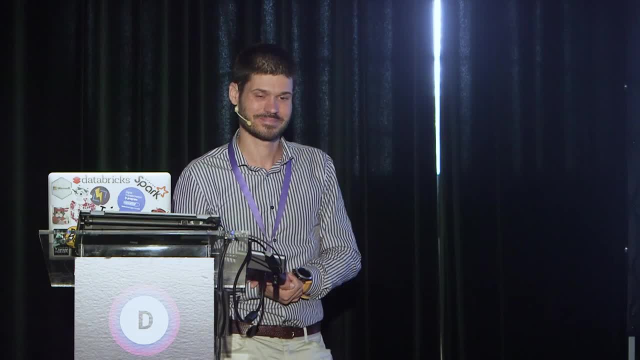 Please, I hope you can handle it. So, for example, our company have already- you know, our company have already- two kind of softwares or what is offered at global deal. One is Cloudera data science workbench. 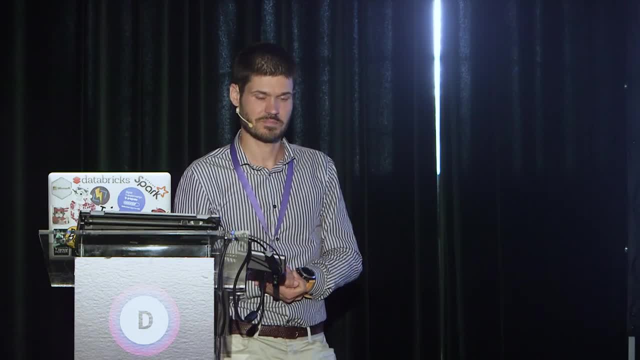 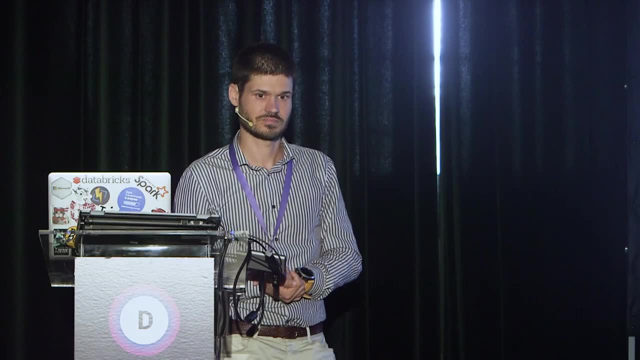 So it's completely based on Jupyter, Notebook or R or Scala, and also supported by the big data infrastructure. Another is a right-pin miner. so basically, one version for non-coding people, another version for hardcore data scientists. So the things that you know, every company. 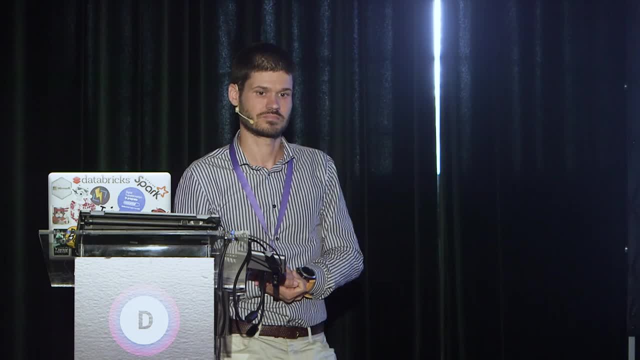 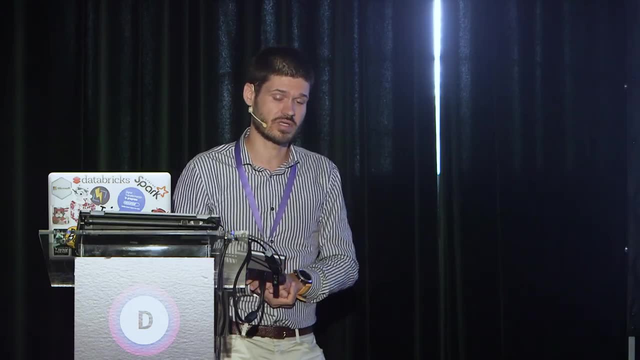 have their own deal. What is your competitive advantage comparing to, you know, Cloudera or rapid miner? So, firstly, Cloudera is a big partner of Microsoft for a long time and there's customers who are running Cloudera large clusters on top of Azure. 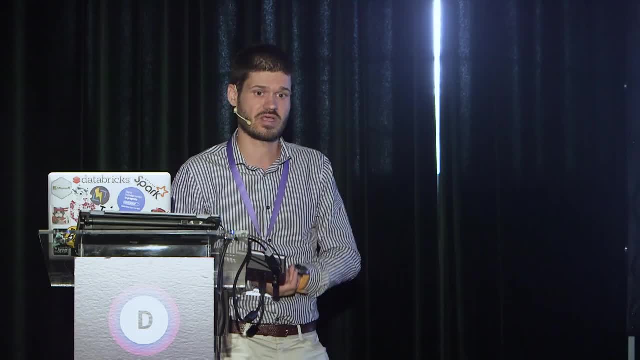 So I will not say it's just either one or the other one. I think if you are existing Cloudera investments with happy parties, you are happy to leverage that in the cloud. The good fact is that you will be able to scale up your cluster. 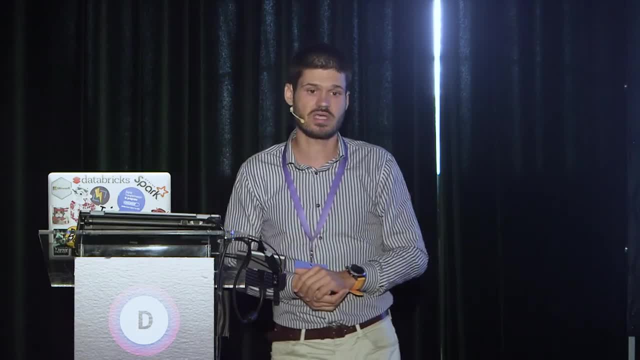 or shut it down. That's already a big advantage. Second thing I will say is we've been, as you've seen, with some of the features I write, we've been investing hard. We've been investing hard to bring cutting-edge features. 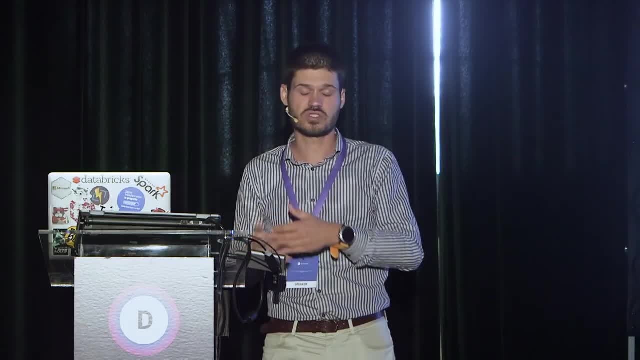 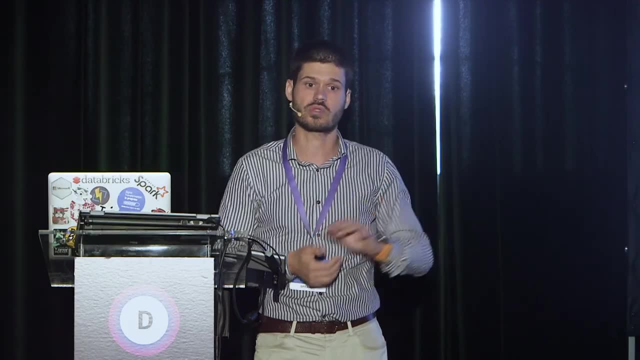 such as graphical experience for non-professional data scientists, open source SDK for any framework, automated machine learning and a few other things that I mentioned. So those ones- I think they are very differentiated to what has been done, probably in the last five years. 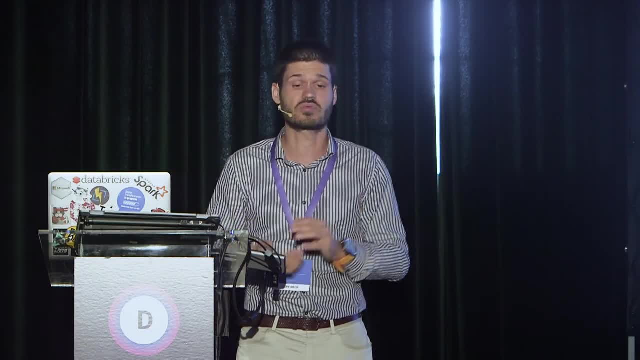 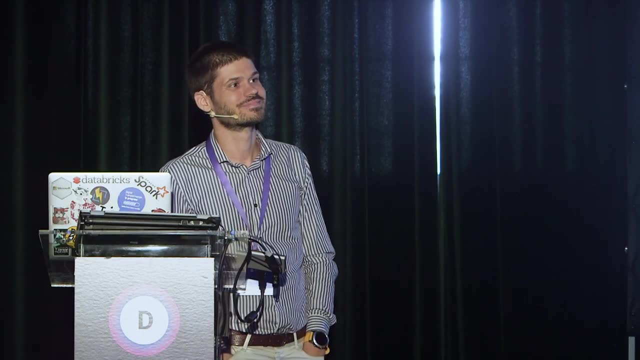 in the market. So I think you have the, you're open to choose both and they have customers using both, which I think is also a sweet spot. So thank you for a great presentation. Thank you, I've never used any automated ML tools, but I'm curious: how do? 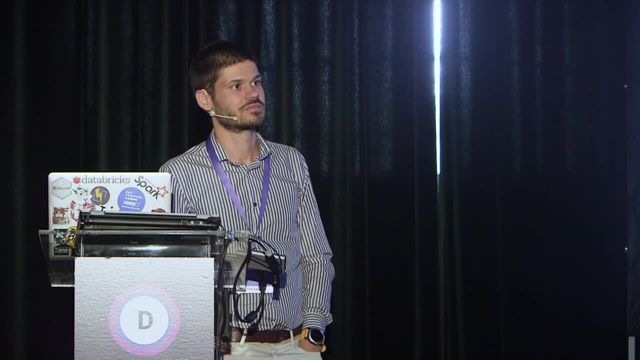 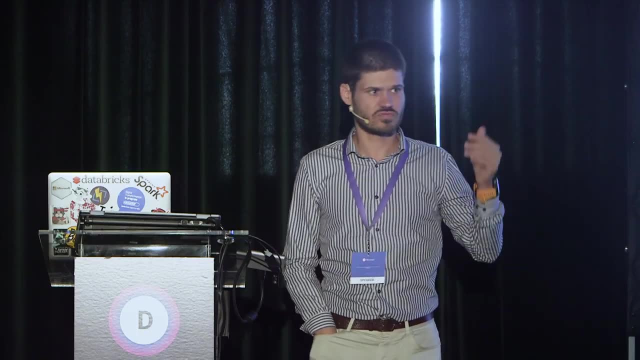 you do hyper-parameter tuning for these kind of automated tools. Yeah, so I didn't go too much into detail. There's three ways you can use AutoML, the one you've seen. Sorry, I cannot see you, but hopefully you can hear me. 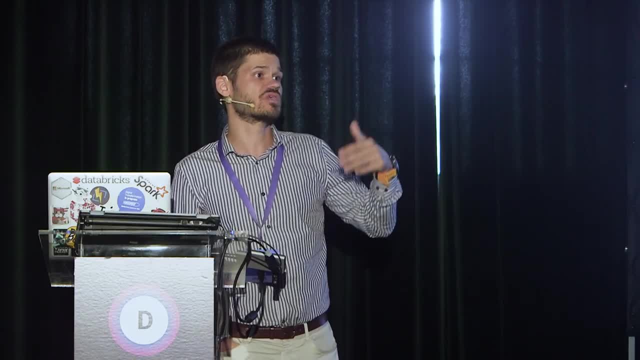 The first one is the basic one. you've seen, It's a graphical one, So it allows you to choose a few things, not more. You don't go to a lot of detail into the hyper-parameters, It's just really to get started. 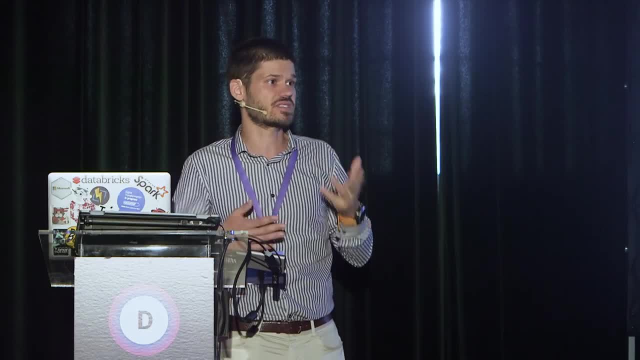 The second way to consume it, which, of course, is the one I prefer, is using the SDK. So that case, you are coding a little bit, so you're specifying a lot more Well parameters to a function, which might be the definition of: how do you? 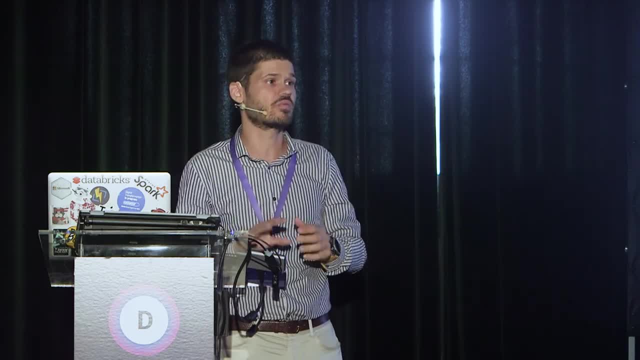 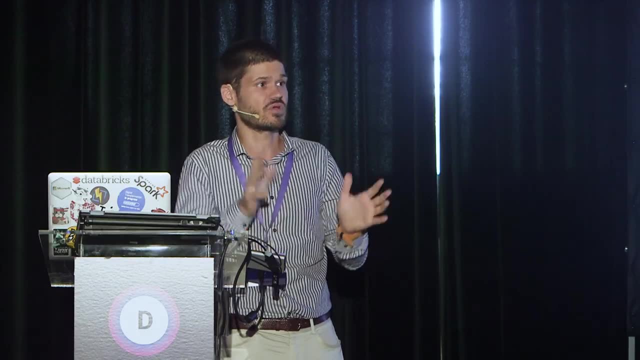 want to play with hyper-parameters. And the third way is basically on Power BI, which is even more business, user-oriented, which you just basically tell what you want to predict and what are the variables, and it does everything for you. So you have the two ways from very basic.